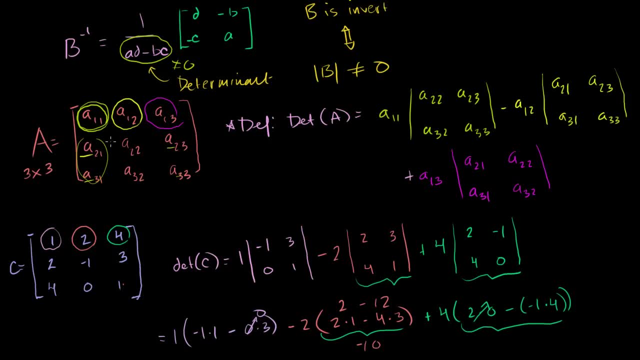 the determinant if you remove his column and his row. So it was left with these terms right there to get that determinant. then finally you switch signs again. So plus this guy times the determinant of the 2 by 2 matrix if you get rid of this row and this column. 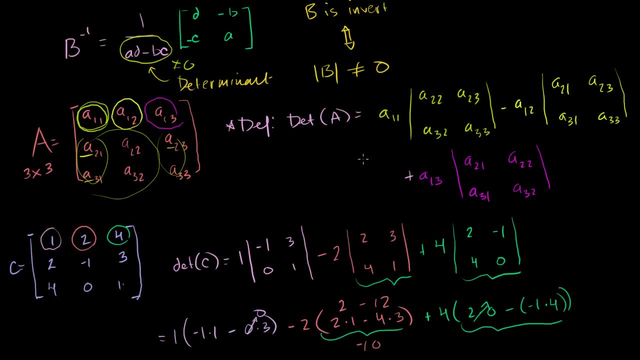 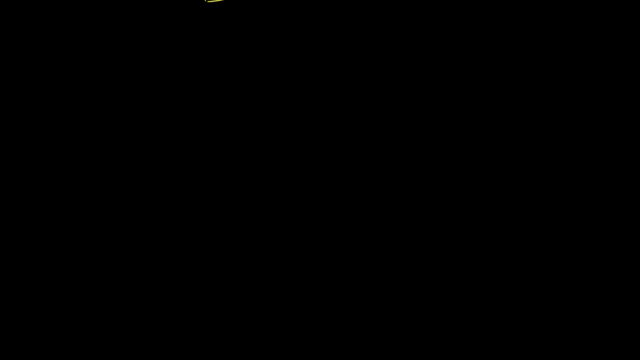 So it's this thing right here which was this matrix. Now let's see if we can extend this to a general n by n matrix. So let's write out our n by n matrix right over here, Do it in blue. So let's say I have some matrix A, that is an n by n matrix. 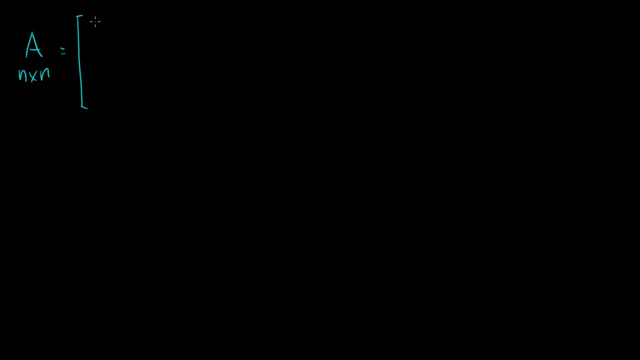 So it's going to look like this: This would be A1- 1,, that would be A1- 2, and it would go all the way to. you're going to have n columns, A1- n, And when you go down, 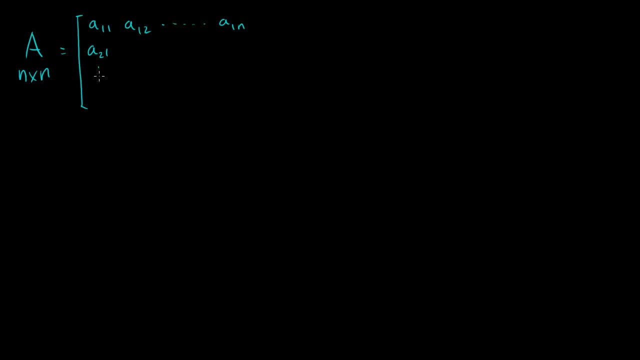 This is going to be your second row, A2- 1.. It's going to go all the way down to AN1, because you have n rows as well, And then, if you go down the diagonal all the way, this right here would be ANN. 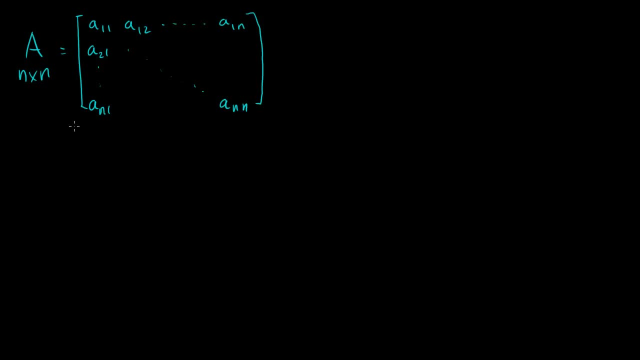 So there is my n by n matrix. Now, before I define how to find the determinant of this, let me make another definition. So this is my matrix A. Let me define A sub-matrix. AIJ to be equal to this is n by n, right. 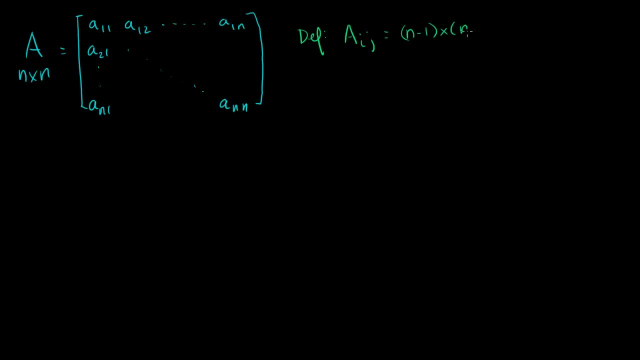 So this is going to be an n minus 1 by n minus 1 matrix. So if this is 7 by 7, the sub-matrix is going to be 6 by 6, one less in each direction. So this is going to be the n minus 1 by n minus 1 matrix. 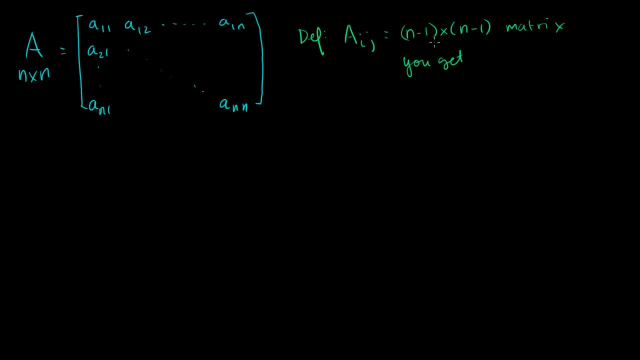 you get. You get If you essentially ignore. If you essentially ignore, If you ignore or if you take away- Maybe I should say take away. When I say ignore, I like the word ignore- If you ignore the ith row, this right here is the row. 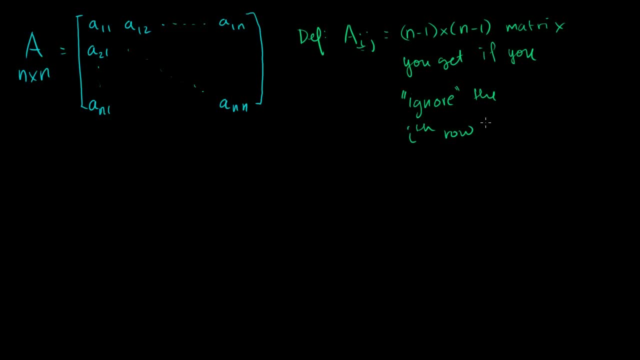 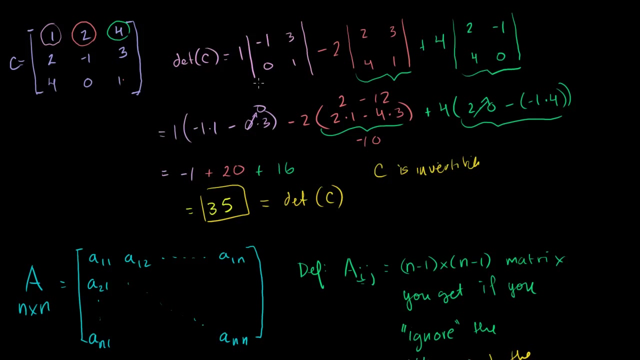 the ith row and the jth column of A. So, for example, let's go back to our 3 by 3.. Right here, This thing could be denoted based on that definition. We could have called this: this was A11, this term right here. 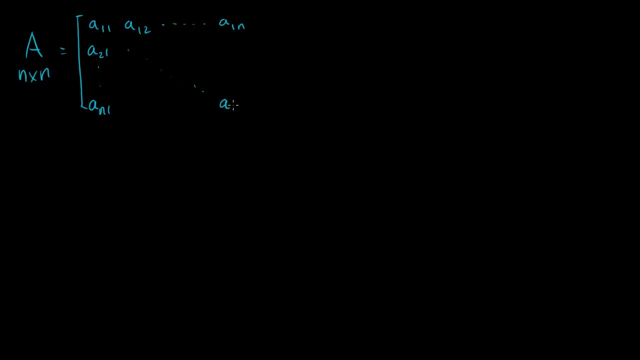 And then if you go down the diagonal all the way, this right here would be Ann. So there is my n by n matrix. 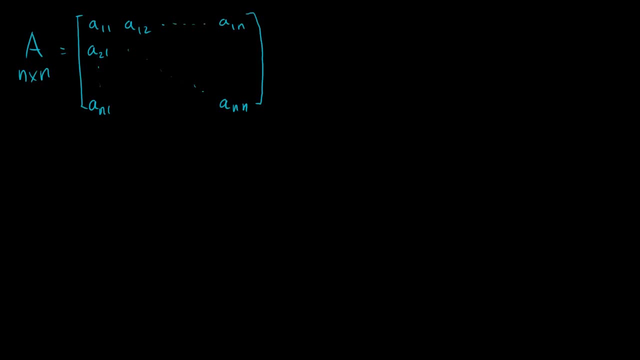 Now, before I define how to find the determinant of this, let me make another definition. So this is my matrix A. Let me define. 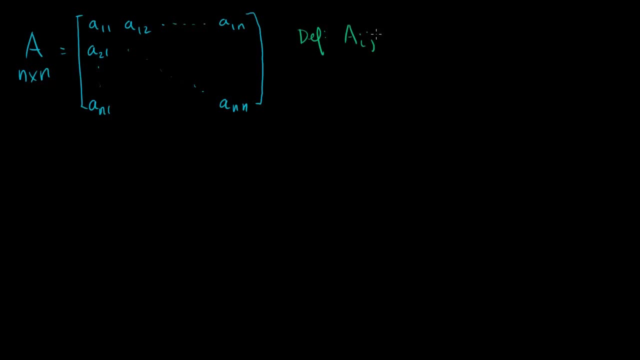 A submatrix, Aij, to be equal to, this is n by n, right? So this is going to be an n minus 1 by n minus 1 matrix. So if this is 7 by 7, the submatrix is going to be 6 by 6, one less in each direction. So this is going to be the n minus 1 by n minus 1 matrix you get, you get, you get, if you essentially ignore, if you ignore, or if you take away, maybe I should say take away, let's say ignore, I like the word ignore. 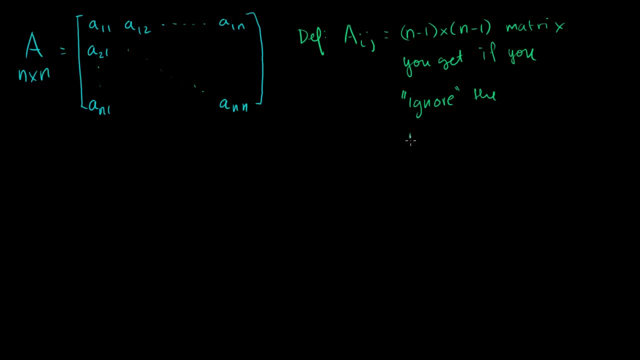 If you ignore the ith row, this right here is the row, the ith row and the jth column of A. 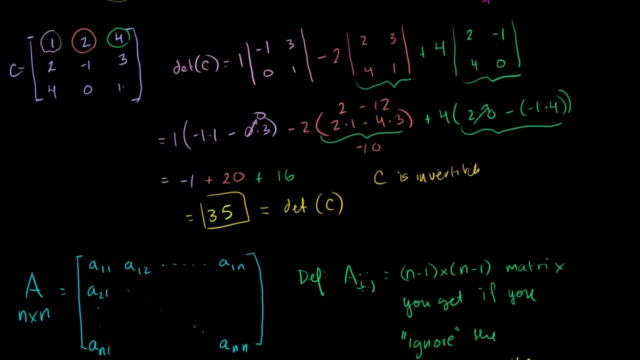 So for example, let's go back to our 3 by 3 right here. 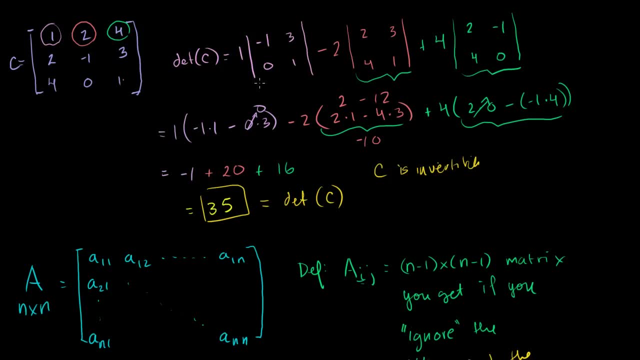 This thing could be denoted, based on that definition, we could have called this, this was A11, this term right here. We could denote the matrix when you get rid of the first column in the first row, or the first row in the first column, we could call this thing right here, we could call that big matrix A11. 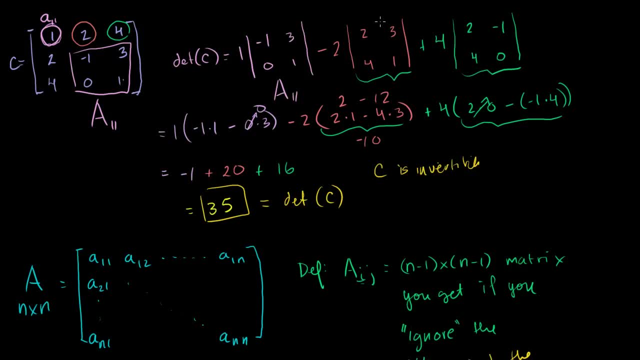 So this was big matrix A11. This is big matrix A21, or actually this matrix was called C. 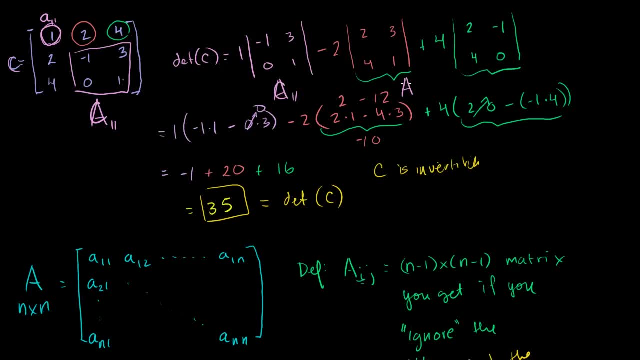 So this would be C11, this would, right there, C11. 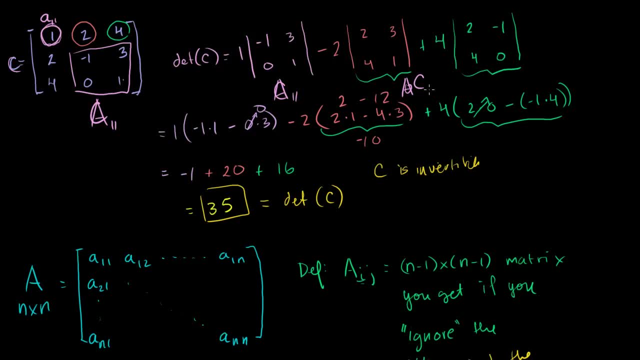 We could call this one, this would be matrix CC12. Why is that? 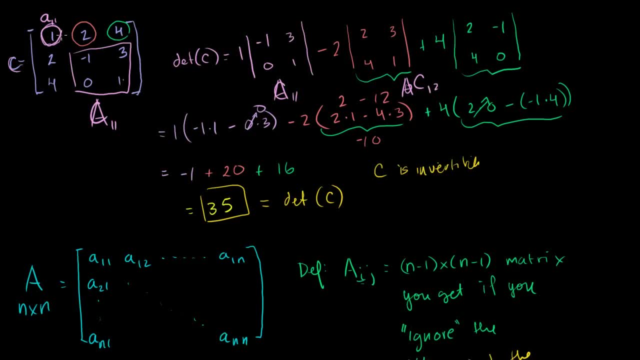 Because if you get rid of the first row, if you get rid of the first row, let me get rid of the first row. Right? The first term is your row. 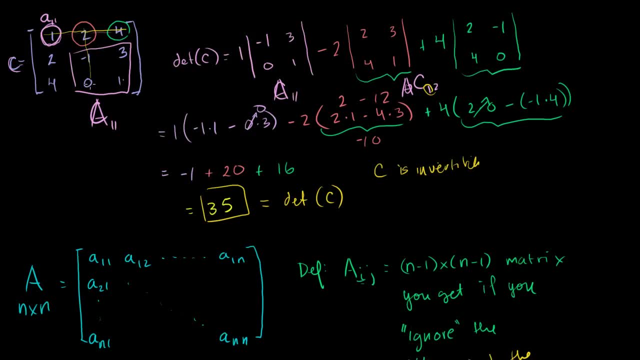 If you get rid of the first row and the second column, this is 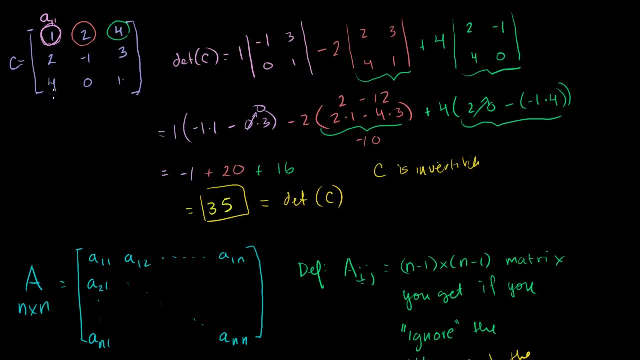 We could denote the matrix when you get rid of the first column and the first row, or the first row and the first column. we could call this thing right here. we could call that big matrix A11.. So this was big matrix A11.. 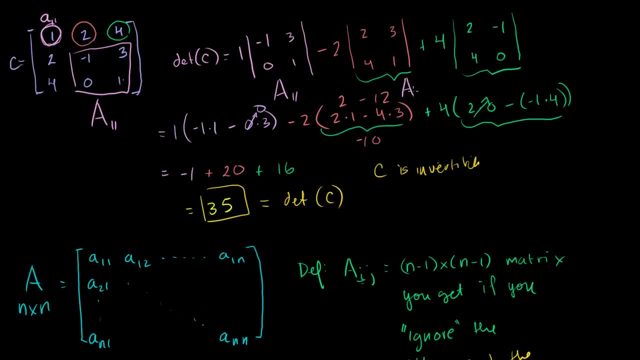 This is big matrix A21.. Or actually, this matrix A21.. This is big matrix A21.. This is big matrix A21.. Or actually, this matrix A21.. This matrix was called C, So this would be C11, right there, C11. 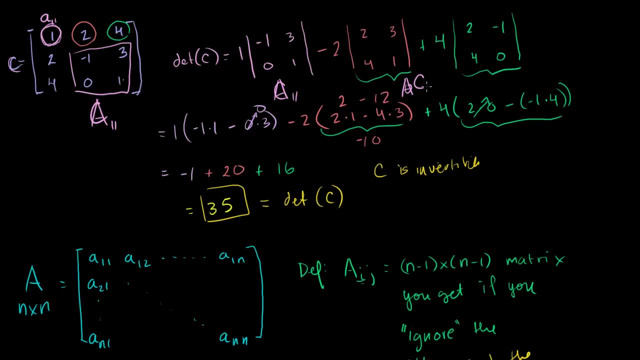 We could call this one. this would be matrix C12.. Why is that? Because if you get rid of the first row, let me get rid of the first row. The first term is your row. If you get rid of the first row and the second column, 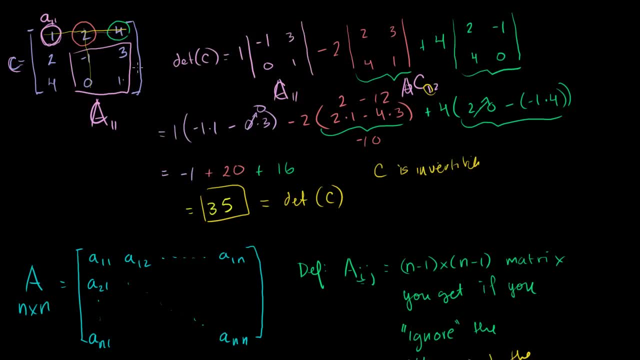 this is the matrix that's left over: 2, 3, 4, 1.. This is this guy and this guy: 2, 3, 4, 1.. So this is the submatrix C, because this: 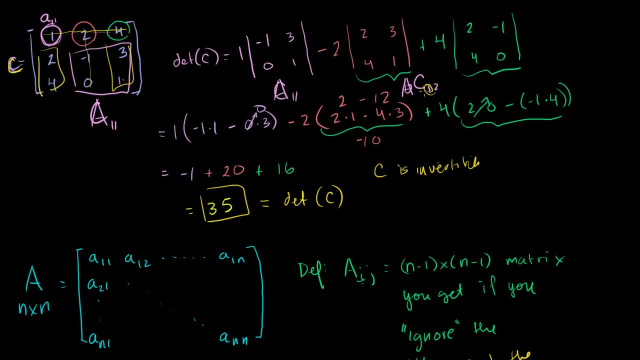 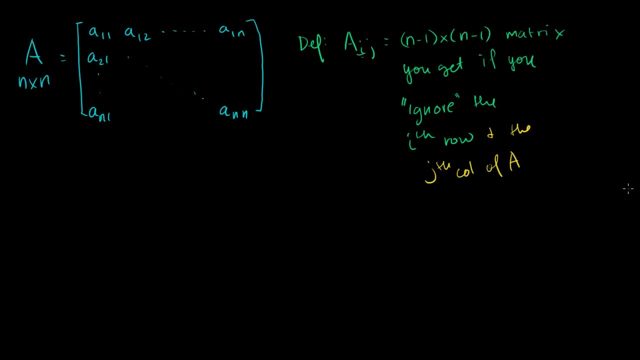 is the big matrix C, But this one is C12.. I know it's a little bit messy there, So that's all we mean by the submatrix, Very similar to what we did in the 3 by 3 case You essentially get rid of. so if you want to find out, 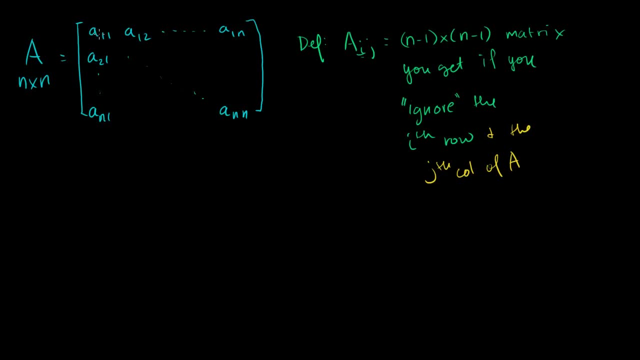 this guy's submatrix. you would call that A11. And you would literally cross out the first row and the first column And everything left over here would be that submatrix. Now, with that out of the way, we can create a definition. 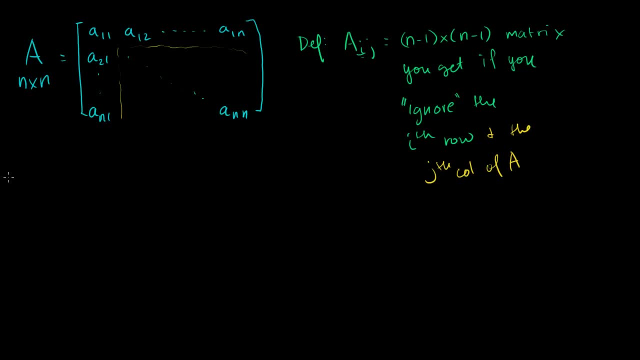 And it might seem a little circular to you at first, And on some level it is. We're going to define the determinant of A to be equal to- and this is interesting- It's actually a recursive definition. I'll talk about that in a second. 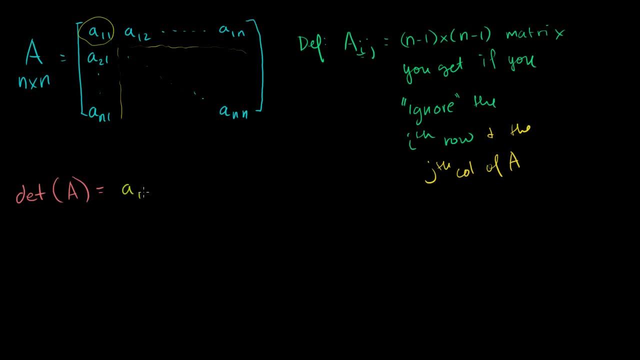 We start with a plus, It's equal to A11 times the submatrix. So if you remove this guy's row and column, So that by definition is just A big capital, A 11's determinant. So that's exactly what we did. 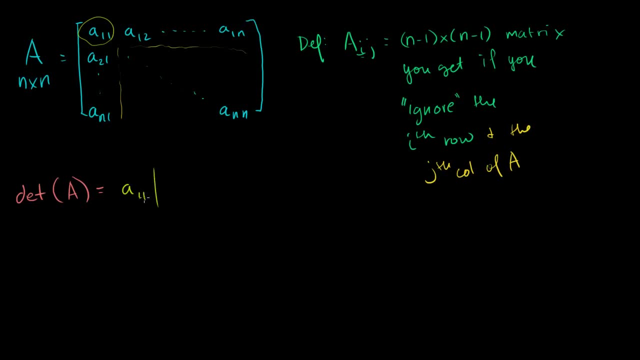 Let me write that a little bit neater: So times the determinant of its submatrix, So the determinant of A11.. So you take A11, you get rid of its column and its row, or its row and its column and everything else. 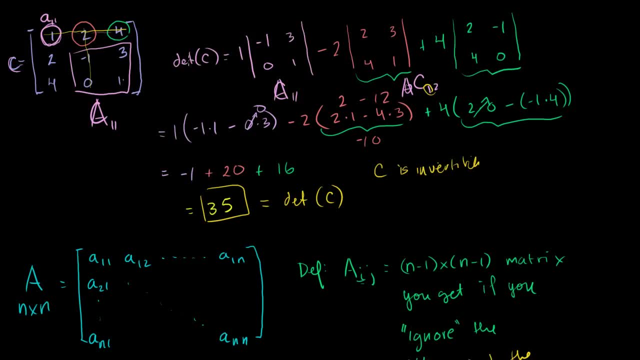 the matrix that's left over. 2, 3, 4, 1. So this is this guy. 2, 3, 4, 1. So this is this guy. So this is this guy. 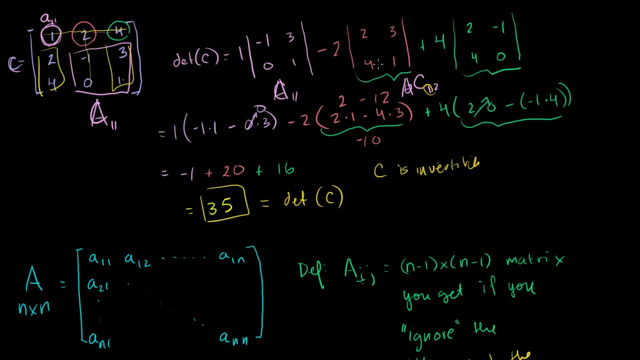 And this guy, 2, 3, 4, 1. So this is the submatrix C, because this is the big matrix C. 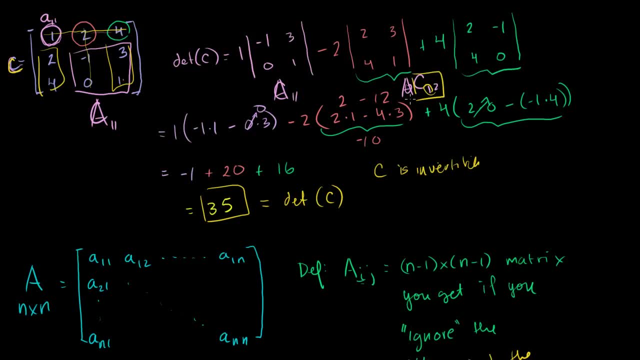 But this one is C, 1, 2. I know it's a little bit messy there. C, 1, 2. 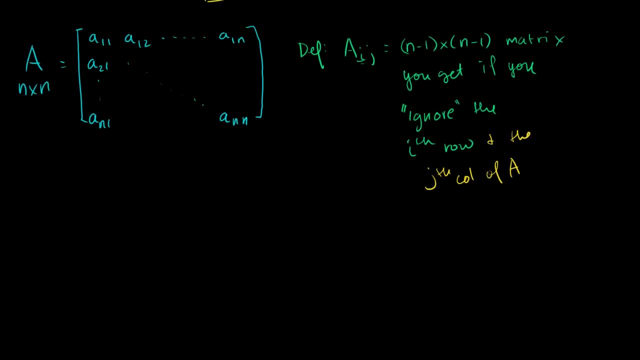 So that's all we mean by the submatrix. Very similar to what we did in the 3 by 3 case. You essentially get rid of, so if you want to find out this guy's submatrix, you would call that A, 1, 1. And you would literally cross out the first row and the first column, and everything left over here would be that submatrix. 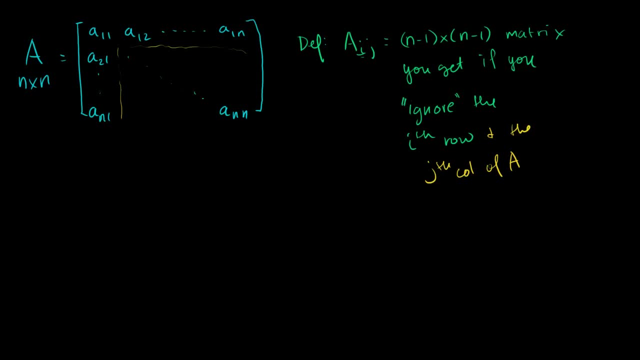 Now, with that out of the way, we can create a definition. And it might seem a little circular to you at first. And on some level, it is. 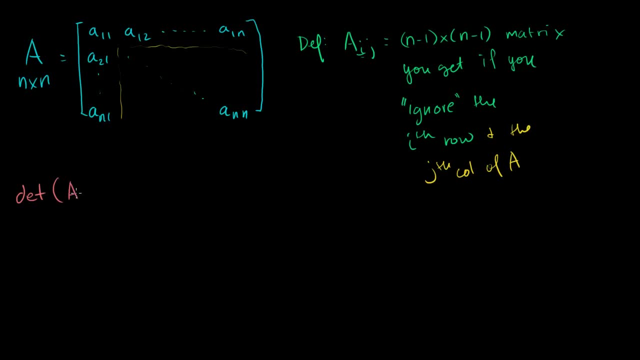 We're going to define the determinant of A to be equal to, and this is interesting. It's actually a recursive definition. I'll talk about that in a second. We start with a plus. It's equal to A, 1, 1. 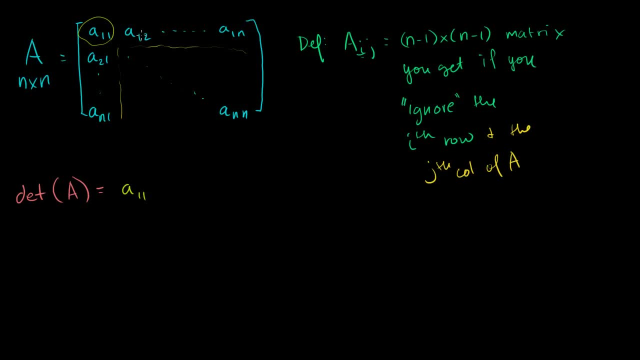 Times the submatrix. Submatrix, if you remove this guy's row and column. 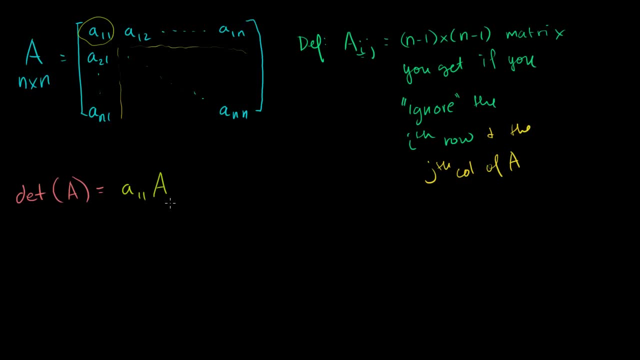 So that, by definition, is just A, big capital A, 1, 1's determinant. 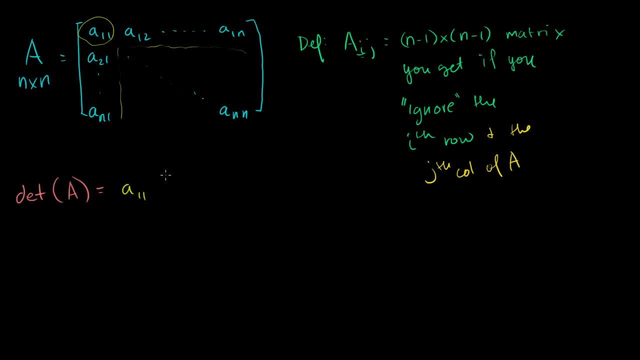 So that's exactly what we did. Let me write that a little bit neater. So times the determinant of its submatrix. 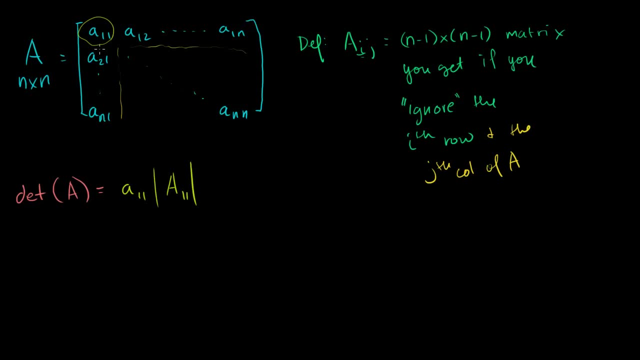 So the determinant of A, 1, 1. So you take A, 1, 1. 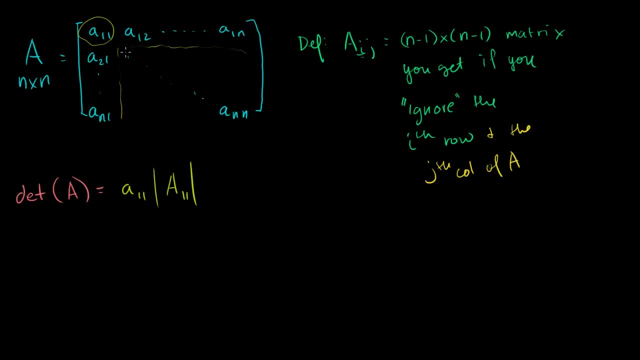 You get rid of its column and its row, or its row and its column, and everything else, you find the determinant of that. 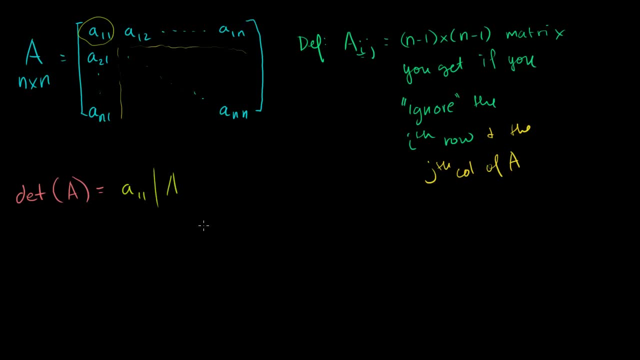 you find the determinant of that. Actually, let me write it in terms of: let me write it this way: A11 times the determinant of the submatrix A11.. And then we switch sides. We're just going to go along this row. 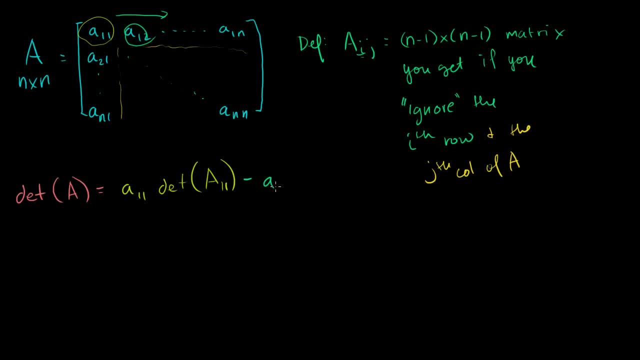 We're just going to go along this row And then you do minus A12 times the determinant of its submatrix, which we'll just call A12.. We would get rid of this row and this column and everything left would be this matrix, A12.. 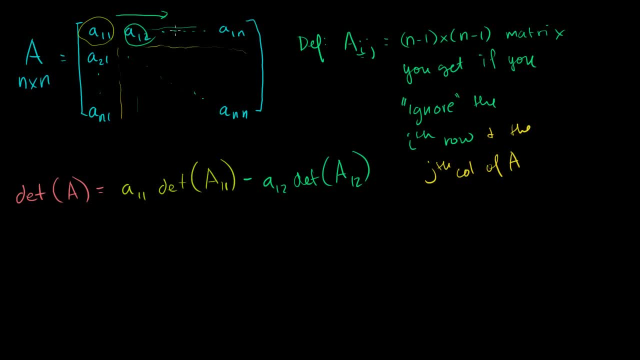 We want to find its determinant, And then we'll take the next. The next guy over here would be A13.. So we switch sides. with minus, Now you go plus. So A13 times the determinant of its submatrix. So these are, if this is n by n each. 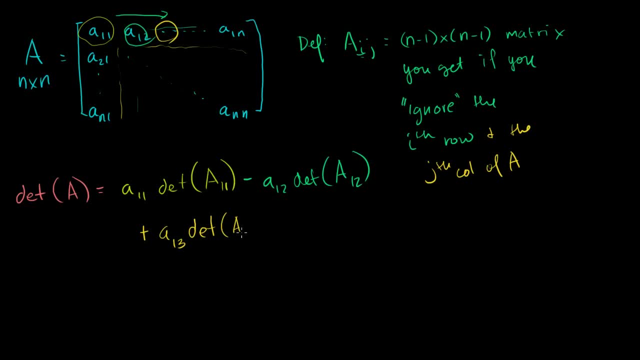 are going to be n minus 1 by n minus 1.. So the determinant of A13.. And you're just going to keep doing that, keep switching signs. So it's going to be a minus and then a plus, And you keep going all the way. 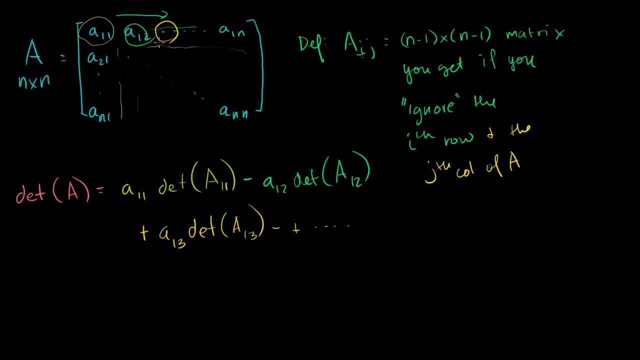 And then I don't know. it depends on whether an whether we're dealing with an odd number or an even number. If we're dealing with an even number, we're going to have to do that. If it's an odd number, this is going to be a minus sign. 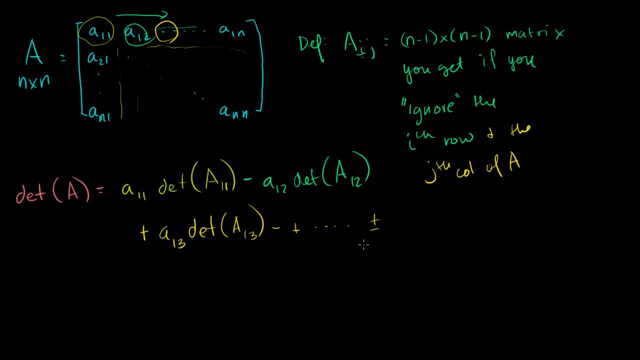 If it's an odd number, it's going to be a plus sign. But you get the idea It's either going to be a plus or a minus. Not just if it's odd, this is going to be a plus. If it's an even n, it's going to be a minus. 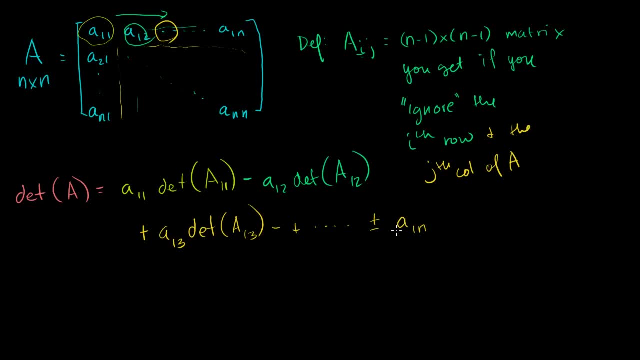 All the way to A1n. the nth column times its submatrix A1n. With that submatrix you get rid of the first row and the nth column and it's going to be everything that's left in between. 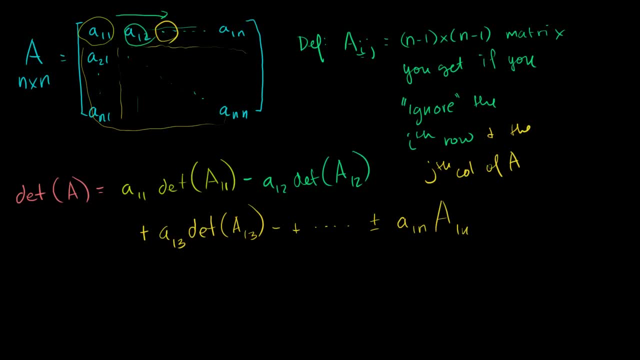 And you immediately might say: Sal, what kind of a definition is this? You've defined a determinant for an arbitrary n by n matrix. in terms of another definition of a determinant, How does this work? And the reason why this works is because the determinants 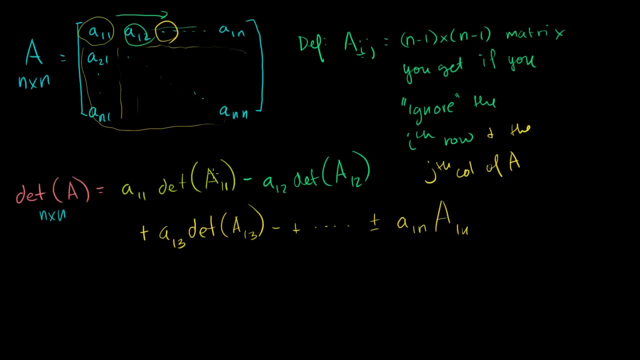 that you use in the definition are determinants of a smaller matrix. So this is a determinant of an n minus 1 by n minus 1 matrix. Now you're saying, hey, Sal, that still doesn't make any sense because we don't know how to find the determinant of. 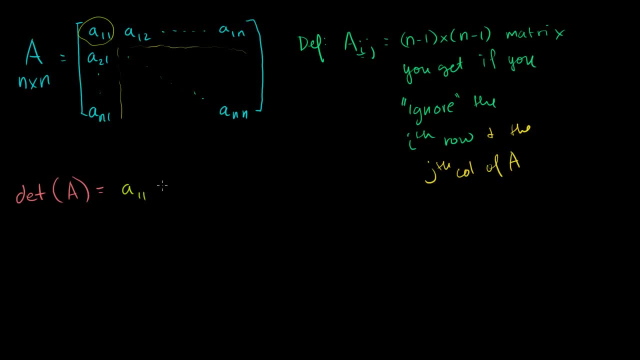 Actually, let me write it in terms of, let me write it this way. A, 1, 1 times the determinant of the submatrix, A, 1, 1. 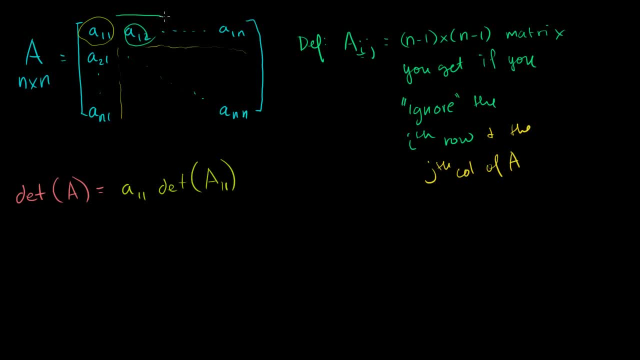 And then we switch sides. We're just going to go along this row. We're just going to go along this row. 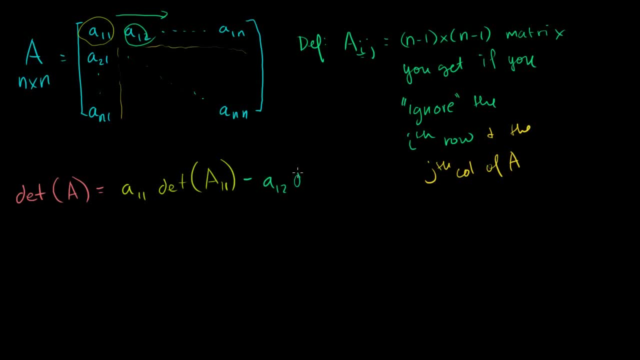 And then you do minus A, 1, 2 times the determinant of its submatrix, which we'll just call A, 1, 2. 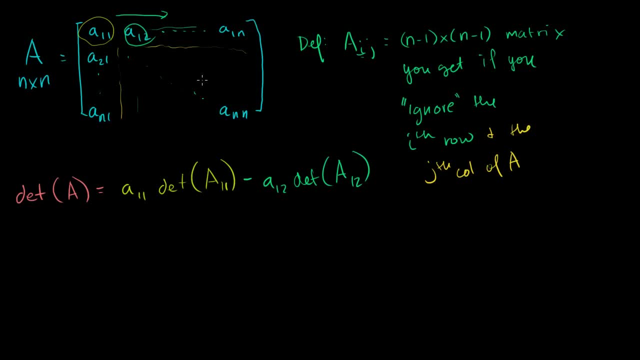 We would get rid of this row and this column, and everything left would be this matrix, A, 1, 2. 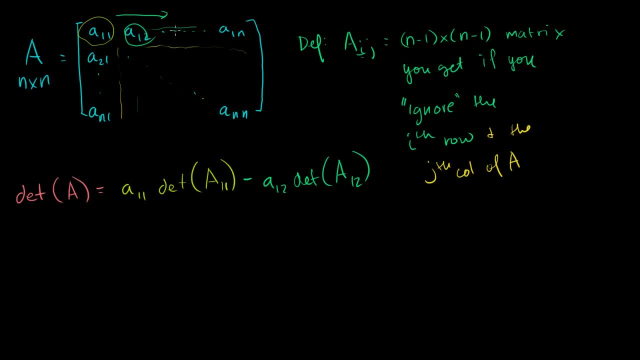 We want to find its determinant. And then we'll take. The next guy over here, who would be A, 1, 3. So we switch sides with minus. Now you go plus. 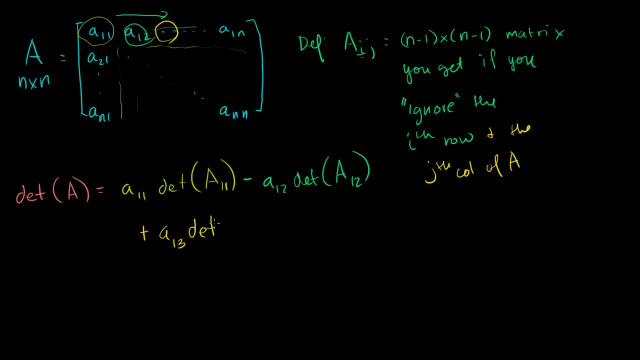 So A, 1, 3 times the determinant of its submatrix. So these are, if this is n by n, these are each going to be n minus 1 by n minus 1. So the determinant of A, 1, 3. And you're just going to keep doing that, keep switching signs, so it's going to be a minus and then a plus. And you keep going all the way. And then, I don't know, it depends on whether A, n, whether we're dealing with an odd number or an even number. If we're dealing with an even number, this is going to be a minus sign. If it's an odd number, it's going to be a plus sign. But you get the idea. It's either going to be a plus or a minus. 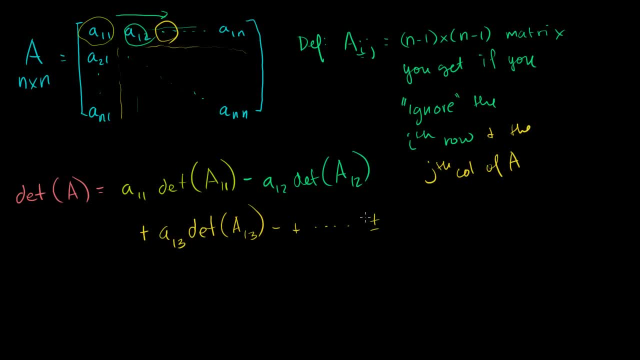 Not just if it's odd, this is going to be a plus. If it's an even n, it's going to be a minus. 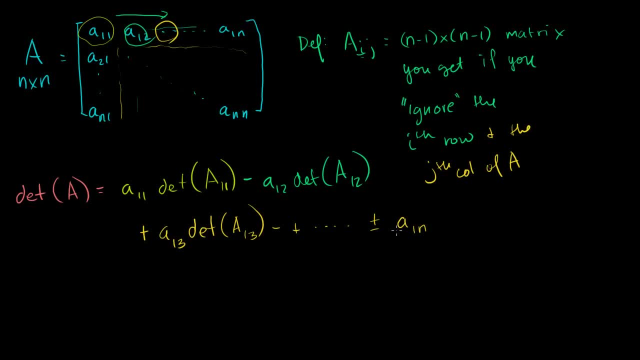 All the way to A, 1, n, the nth column, times its submatrix. A, 1, n. 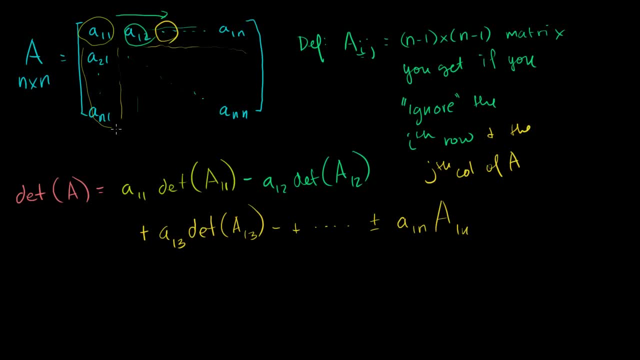 With that submatrix, you get rid of the first row and the nth column, and it's going to be everything that's left in between. And you immediately might say, Sal, what kind of a definition is this? 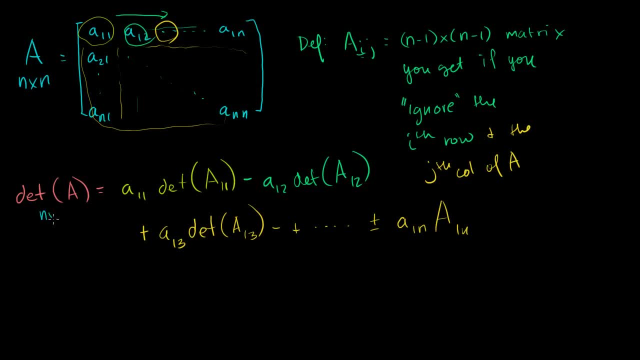 You've defined a determinant for an arbitrary n by n matrix in terms of another definition of a determinant. How does this work? 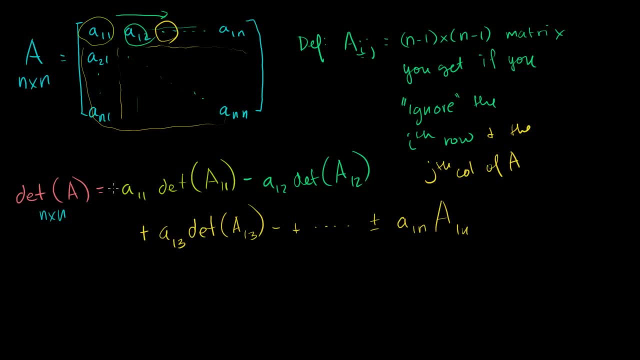 And the reason why this works is because the determinants that you use in the definition are determinants of a smaller matrix. 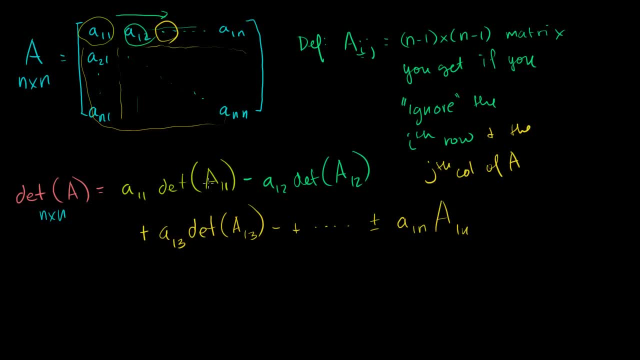 So this is a determinant of an n minus 1 by n minus 1 matrix. And you're saying, hey, Sal, that still doesn't make any sense, because we don't know how to find the determinant of an n minus 1 by n minus 1 matrix. 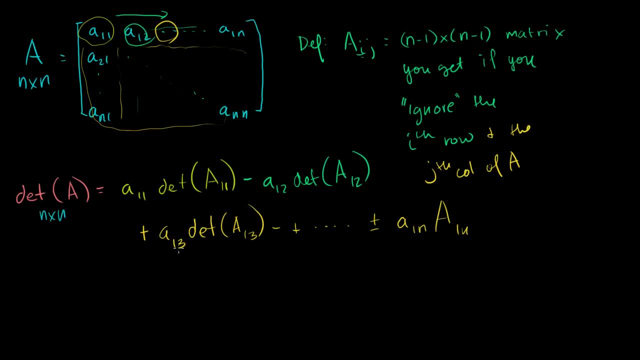 an n minus 1 by n minus 1 matrix. Well, you apply this definition again and then it's going to be in terms of n minus 1.. n minus 2 by n minus 2 matrices. And you're like: how do you do that? 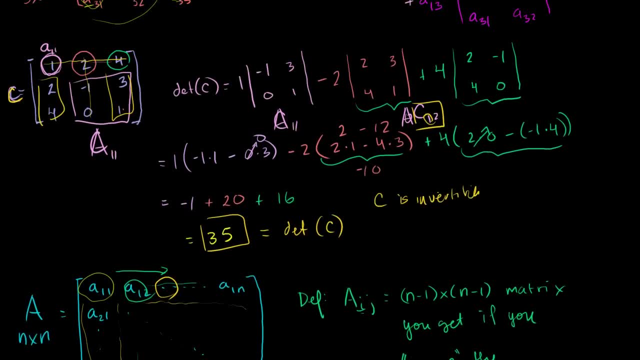 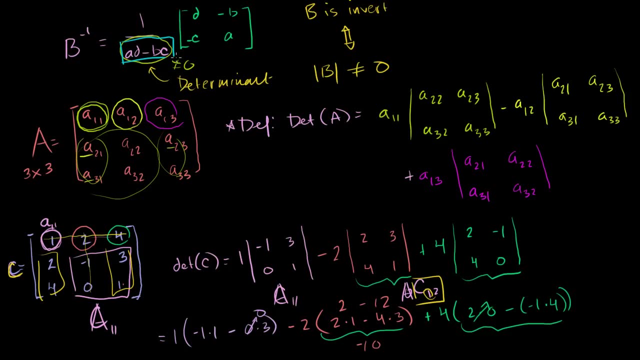 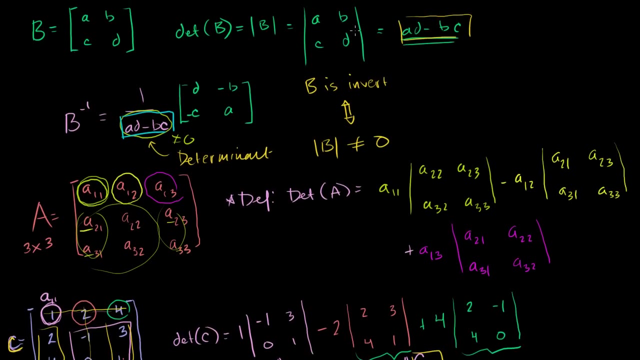 Well, you keep doing it and you're going to get all the way down to a 2 by 2 matrix, And that one we defined. well, We defined the determinant of a 2 by 2 matrix not in terms of a determinant, we just defined it in terms of a times d minus b. 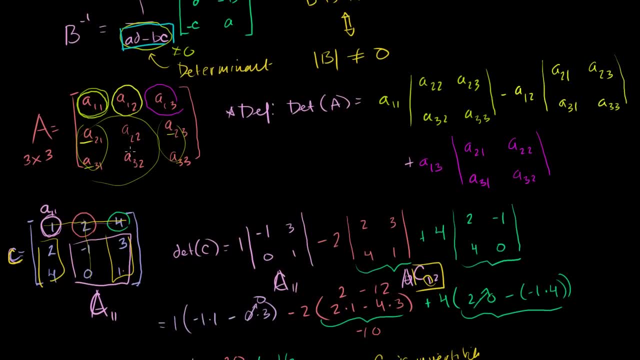 times c And you can see we could just go down to the 3 by 3, but the 2 by 2 is really the most fundamental definition And you could see that the definition of a 3 by 3 determinant is essentially a special case of the general. 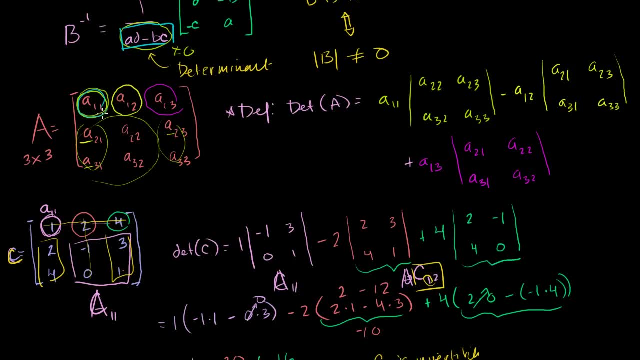 case for an n by n, We take this guy and we multiply him times the determinant of his sub matrix, right there. Then we take this guy, we switch signs, we have a minus and we multiply him times the determinant of his sub matrix. 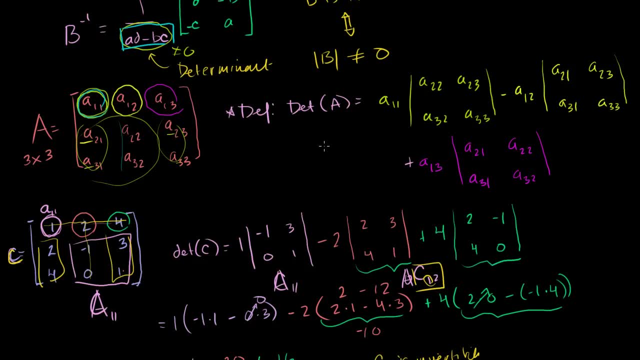 which is that right there. And then you do a plus, You switch signs and then you multiply. this guy times the determinant of his sub matrix, which is that right there. So this is a general case of what I just defined, But we know it's never that satisfying to deal in the 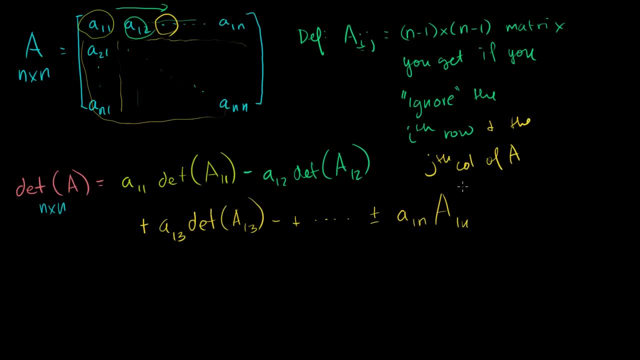 abstract or the generalities. We want to do a specific case And actually, before I do that, let me just introduce a term to you. This is called a recursive formula, And if you become a computer science major, you'll see this. 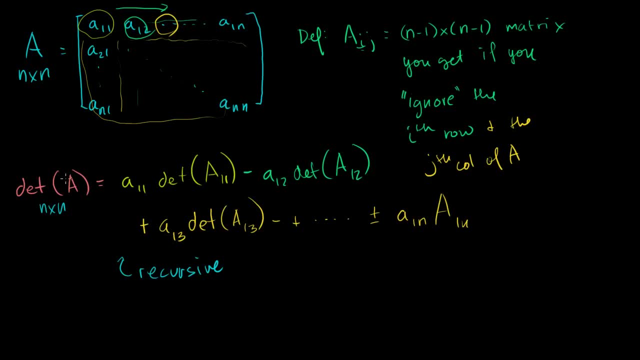 a lot, but a recursive function or a recursive formula is defined in terms of itself, But the things that you use in the definition use a slightly simpler version of it And as you keep going through, you keep recursing through it, you get simpler and 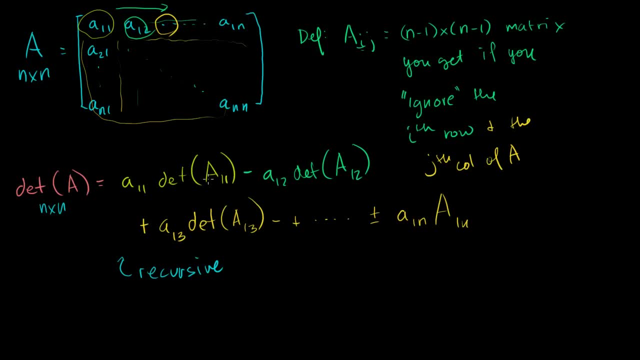 simpler And you get simpler versions of it until you get to some type of base case. In this case, our base case is the case of a 2 by 2 matrix. You keep doing this and eventually you'll get to a determinant of a 2 by 2 matrix. 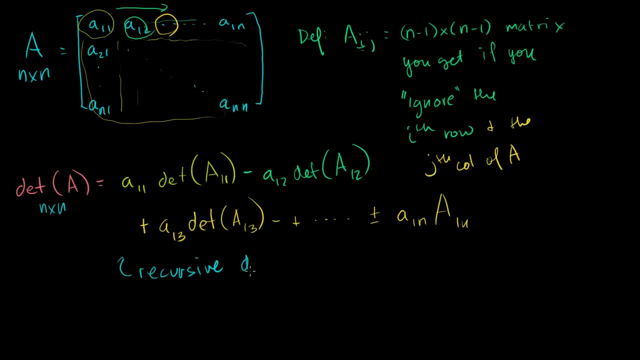 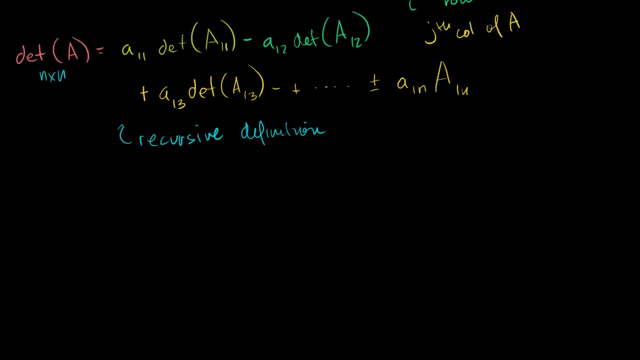 And we know how to find those. So this is a recursive definition, But let's actually apply it, because I think that's what actually makes things concrete. So let's take a. this is going to be computationally intensive, but I think if we focus we can get there. 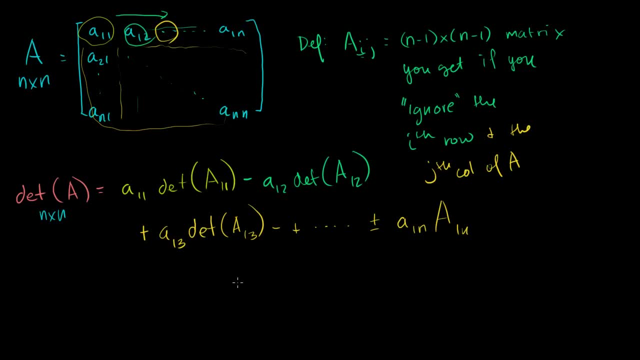 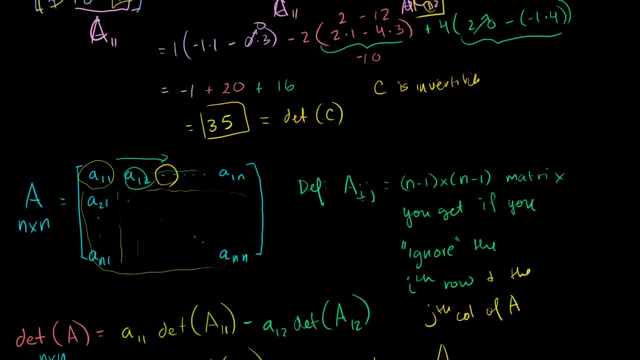 Well, you apply this definition again, and then it's going to be in terms of n minus 2 by n minus 2 matrices. And you're like, how do you do that? Well, you keep doing it, and you're going to get all the way down to a 2 by 2 matrix. 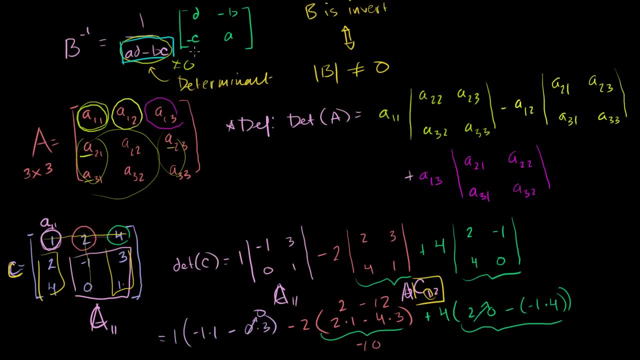 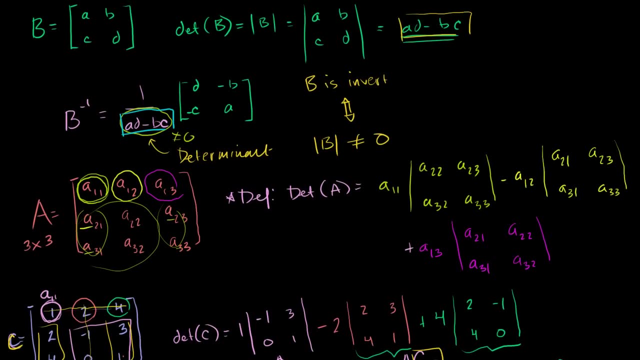 And that one we defined well. We defined the determinant of a 2 by 2 matrix not in terms of a determinant, we just defined it in terms of a times d minus b 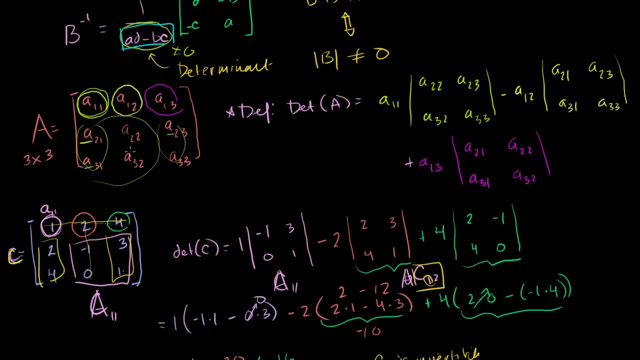 times c. And you can see, we could just go down to the 3 by 3, but the 2 by 2 is really the most 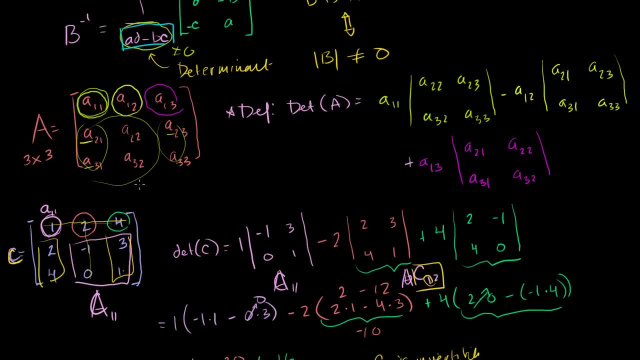 fundamental definition. And you could see that the definition of a 3 by 3 determinant is essentially a special case of the general case for an n by n. 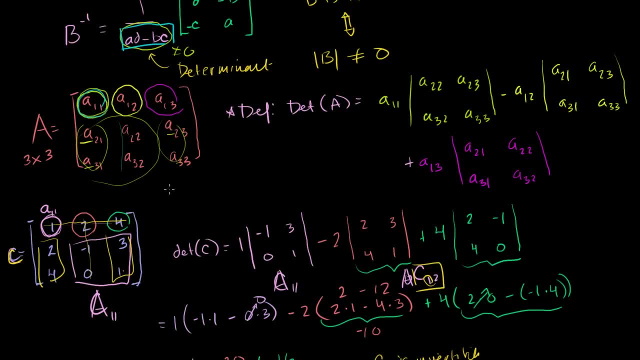 We take this guy, and we multiply him times the determinant of his submatrix right there. Then we take this guy, we switch signs, we have a minus, and we multiply him times the determinant of his submatrix, which is that right there. And then you do a plus. You switch signs, and then you multiply this guy times the determinant of his submatrix, which is that right there. So this is a general case of what I just did. I just defined. 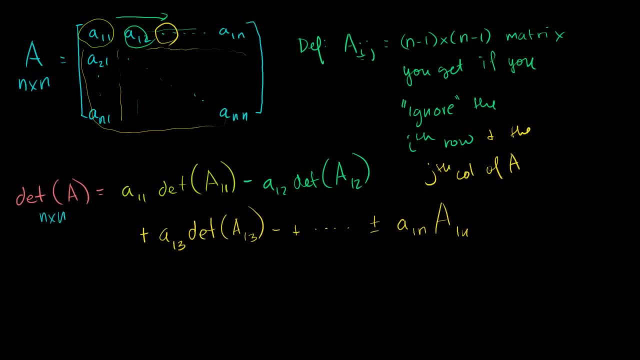 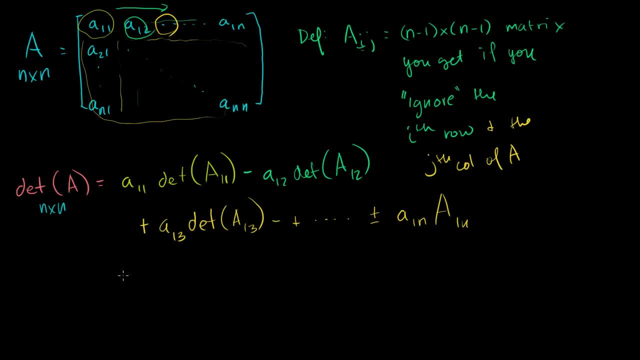 But we know it's never that satisfying to deal in the abstract or the generalities. We want to do a specific case. And actually, before I do that, let me just introduce a term to you. This is called a recursive formula. And if you become a computer science major, you'll see this a lot, but a recursive function or a recursive formula is defined in terms of itself. 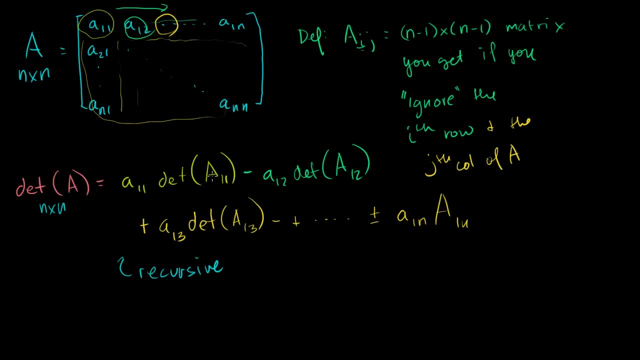 But the things that you use in the definition use a slightly simpler version of it. And as you keep going through, you keep recursing through it, you get simpler and simpler versions of it until you get to some type of base case. In this case, our base case is the case of a 2 by 2 matrix. You keep doing this, and eventually you'll get to a determinant of a 2 by 2 matrix. 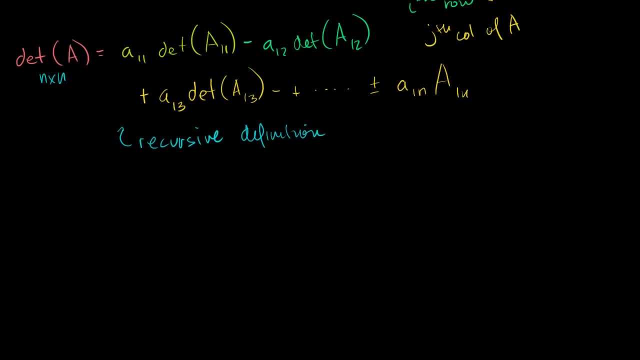 But let's actually apply it, because I think that's what actually makes things concrete. So let's take a, this is going to be computationally intensive, but I think if we focus, we can get there, so I'm going to have a 4 by 4 matrix. 1, 2, 3, 4, 1, throw some 0's in there to make the computation a little bit simpler. 0, 1, 2, 3, and then 2, 3, 0, 0. 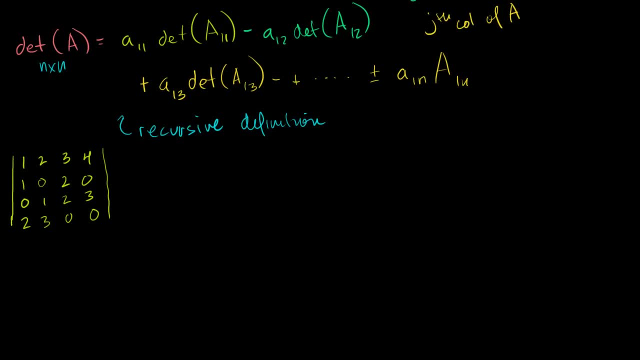 So let's figure out this determinant. Let's figure out this determinant right there. 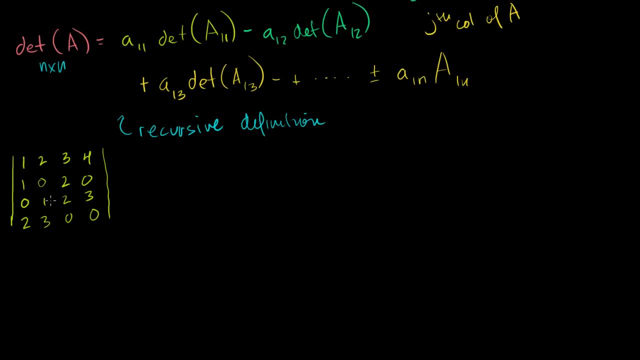 This is the determinant of the matrix. If I put some brackets there, that would have been the matrix, but let's find the determinant of this matrix. So this is going to be equal to, by our definition, it's going to be equal to 1 times the determinant of this matrix right here. If you get rid of this row and this column, so it's going to be 1 times the determinant of 0, 2, 0, 1, 2, 3, 3, 0, 0. That's just this guy right here. 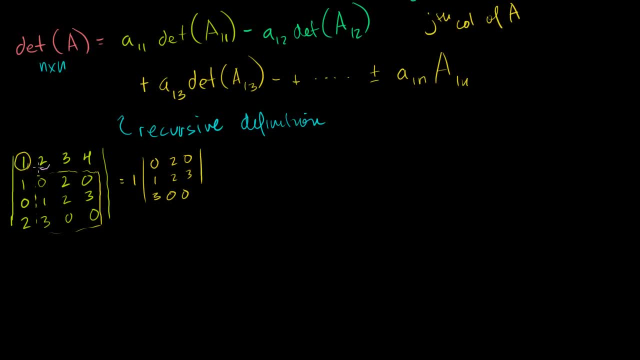 This matrix right there. Then I'm going to have a 2, but I'm going to switch signs. So it's minus 2. Minus 2 times the determinant. If I get rid of that row. If I get rid of that row and this column. So it's 1, 2, 0. I'm ignoring the 0 because it's in the same column as the 2. 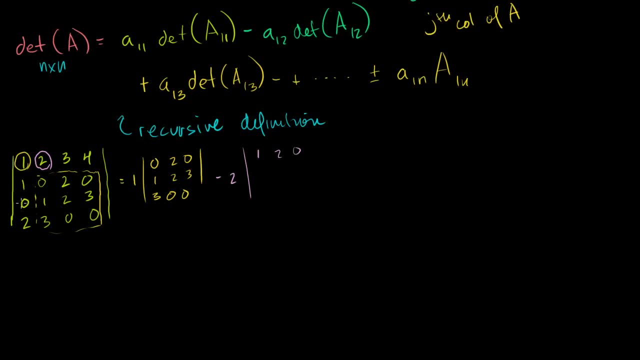 1, 2, 0. So 1, 2, 0. 0, 2, 3. 0, 2, 3. And then 2, 0, 0. 2, 0, 0. 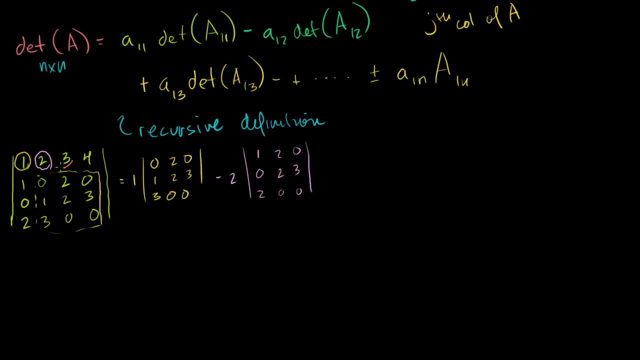 And then I switch signs again. It was a minus, so now I go back to plus. So I do that guy. 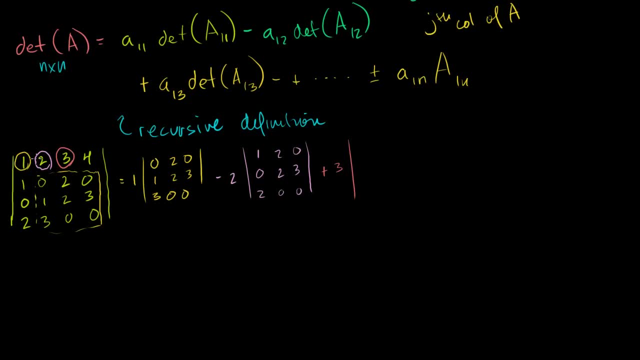 So plus 3 times the determinant of his sub matrix. Get rid of that row. Get rid of that comma. I get a 1, 0, 0. 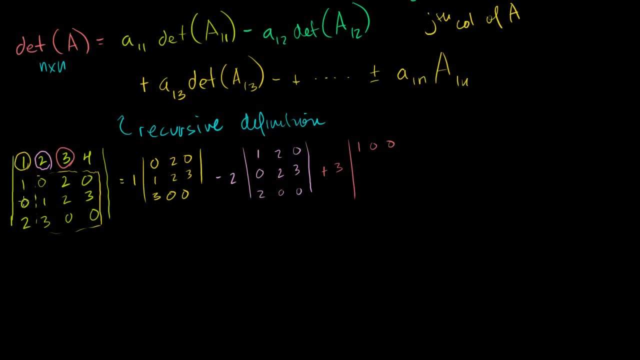 1, 0, 0. I get a 0, 1, 3. 0, 1, 3. 0, 1, 3. I skip this column every time. 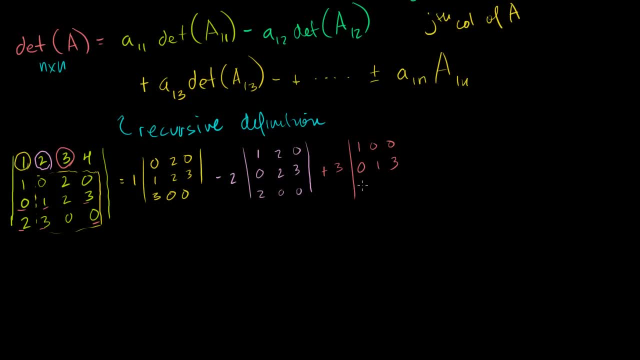 Then I get a 2, 3, 0. 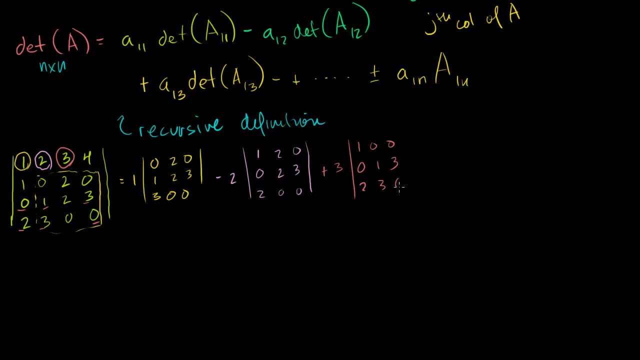 I get a 2, 3, 0. Just like that. 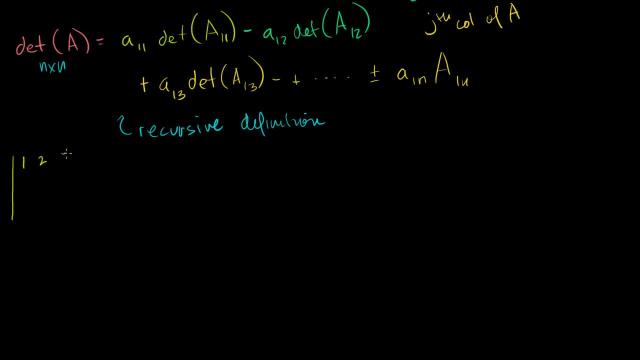 So I'm going to have a 4 by 4 matrix: 1, 2,, 3,, 4, 1, throw some 0's in there to make the computation a little bit simpler: 0, 1,, 2,, 3, and then 2, 3, 0, 0. 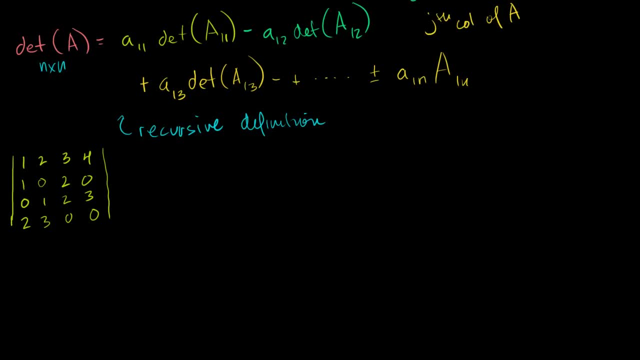 So let's figure out this determinant. Let's figure out this determinant right there. This is the determinant of the matrix. If I put some brackets there, that would have been the matrix, but let's find the determinant of this matrix. So this is going to be equal to 0.. 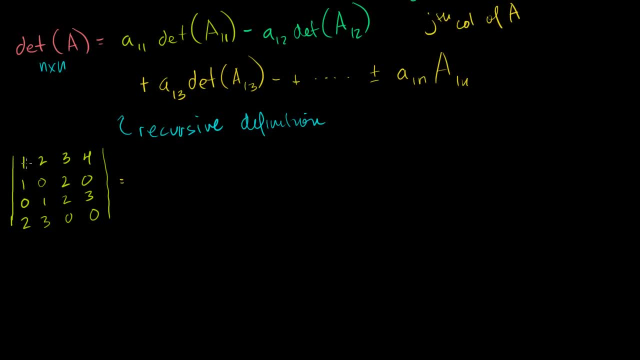 By our definition, it's going to be equal to 1 times the determinant of this matrix. right here, If you get rid of this row and this column, it's going to be 1 times the determinant of 0, 2, 0, 1, 2, 3, 3, 0, 0.. 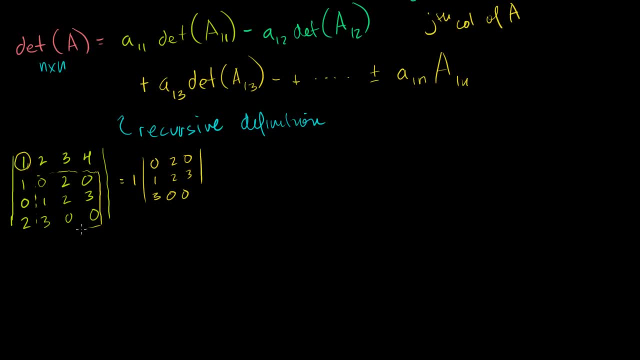 That's just this guy right here, This matrix right there. Then I'm going to have a 2, but I'm going to switch signs, So it's minus 2.. Minus 2 times the determinant if I get rid of that row and 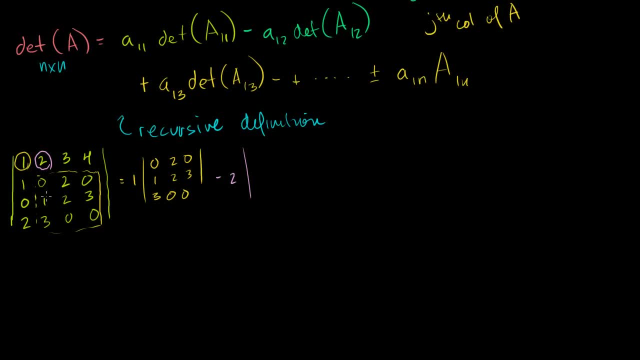 this column. So it's 1, 2, 0.. I'm ignoring the 0 because it's in the same column as the 2.. 1, 2, 0.. So 1, 2, 0.. 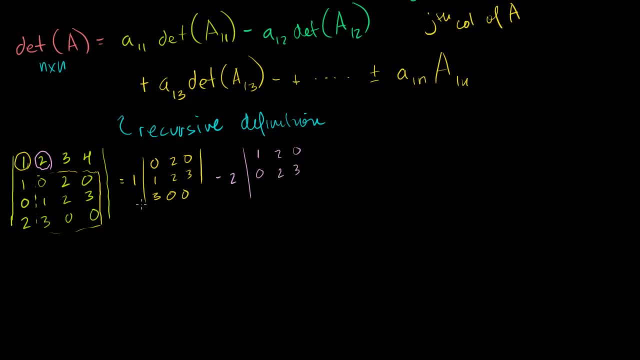 0, 2, 3.. And then 2, 0, 0.. And then I switch signs again. It was a minus, so now I go back to plus, So I do that guy, So plus 3 times the determinant of his sub-matrix. 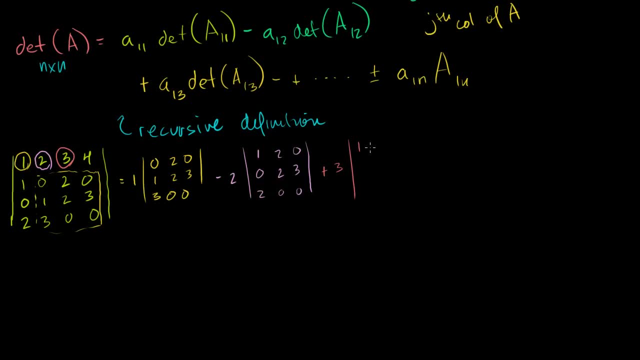 Get rid of that row, Get rid of that column. I get a 1, 0, 0.. 0, 0.. I get a 0, 1, 3.. 0, 1, 3.. 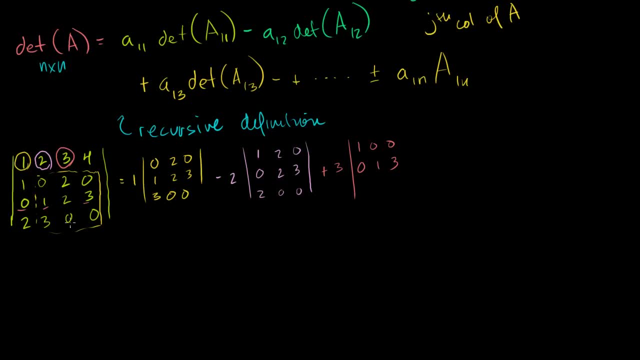 0, 1, 3.. I skip this column every time. Then I get a 2, 3, 0.. I get a 2, 3, 0.. Just like that, We're almost done. One more in this column. 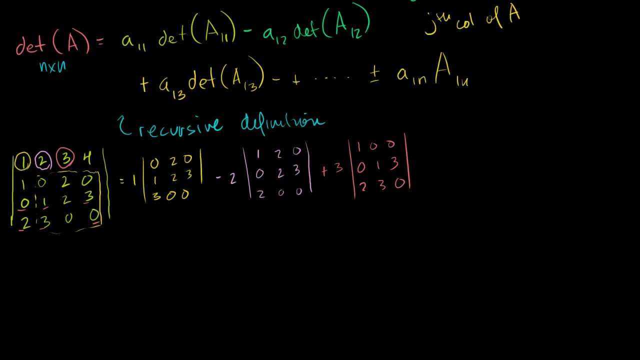 Let me switch to another color. I haven't used the blue in this yet, So then I'm going to do a minus 4.. Remember, It's plus, Minus, plus, minus, 4 times the determinant of its sub-matrix. 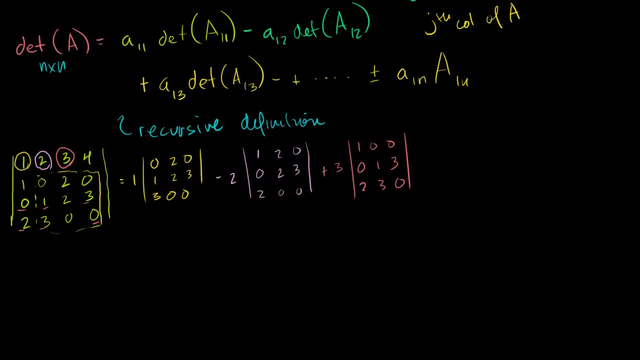 We're almost done. One more in this column. 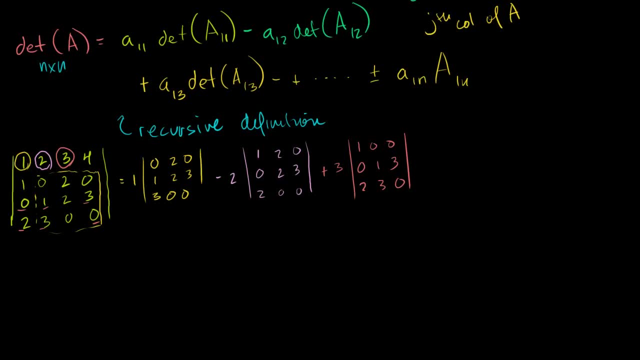 Let me switch to another color. I haven't used the blue in this yet. So then I'm going to do a minus. Minus 4. 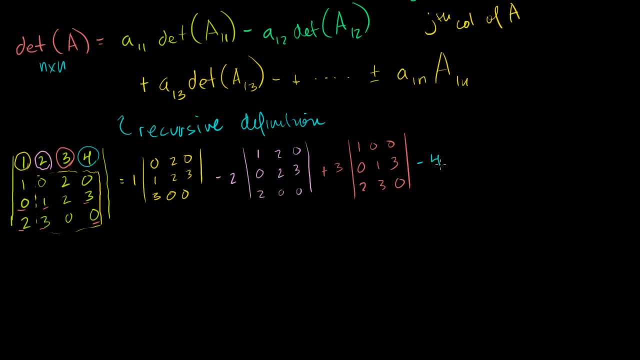 Remember, it's plus, minus, plus, minus 4 times the determinant of its sub matrix. 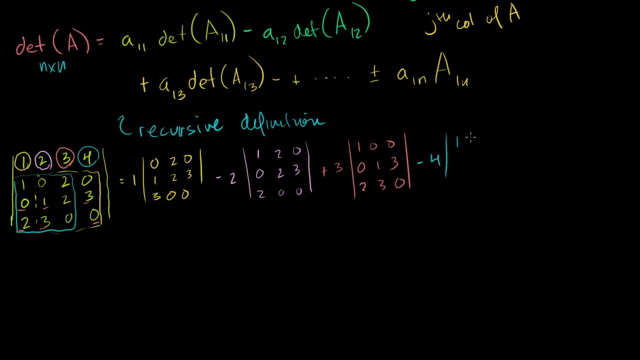 That's going to be that right there. So it's 1, 0, 2. 0, 1, 2. 2, 3, 0. Just like that. 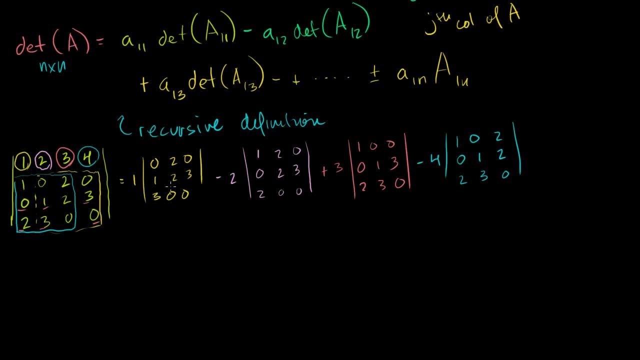 And now we're down to the 3 by 3 case. We could use the definition of the 3 by 3, but we could just keep applying this recursive definition. So this is going to be equal to. Let me write it here. 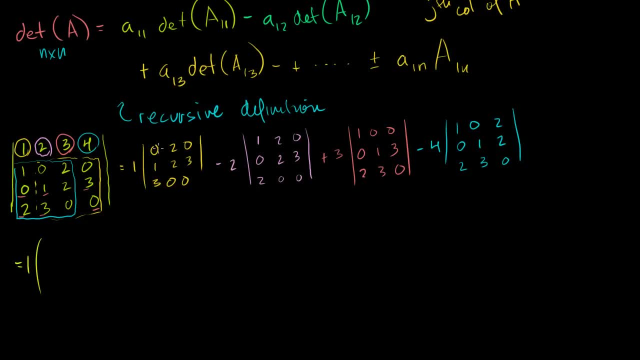 So 1 times, what's this determinant? This determinant is going to be 0. 0 times the determinant of that sub matrix. 2, 3, 0, 0. 2, 3, 0, 0. That was this one right here. And then we have minus 2, minus this 2. 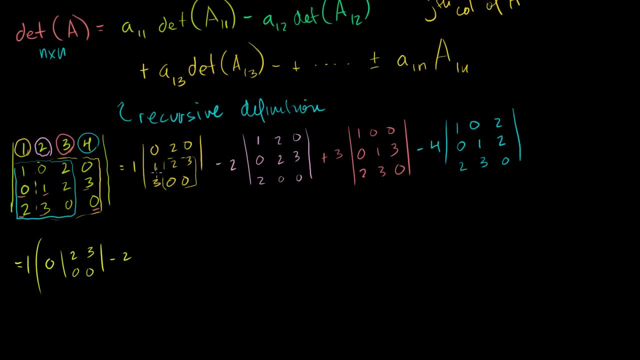 Remember, we switched signs. Plus, minus, plus. So minus 2 times its sub matrix. 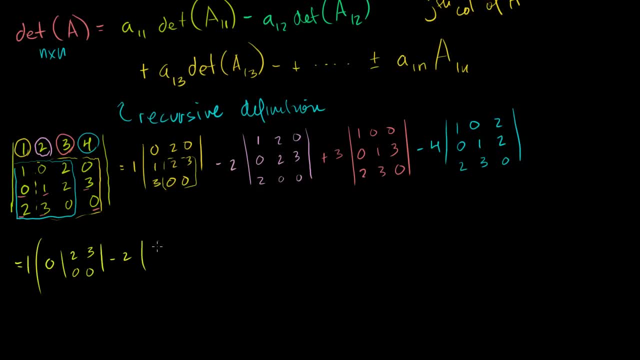 It's 1, 3, 3, 0. 1, 3, 3, 0. 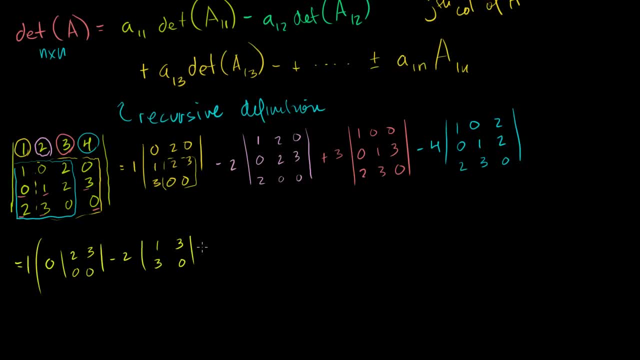 And then, finally, plus 0 times its sub matrix, which is this thing right here. 1, 2, 3, 0. 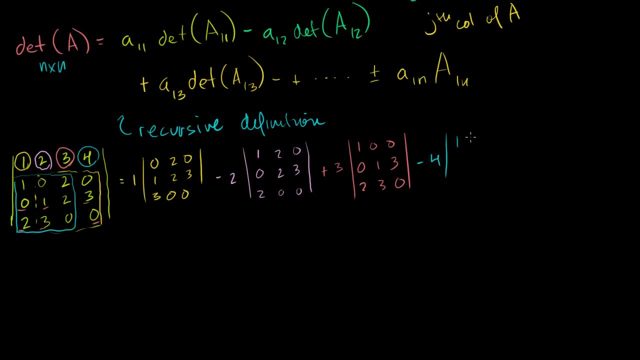 That's going to be that right there. So it's 1, 0, 2.. 0, 1, 2.. 2, 3, 0. Just like that, And now we're down to the 3 by 3 case. 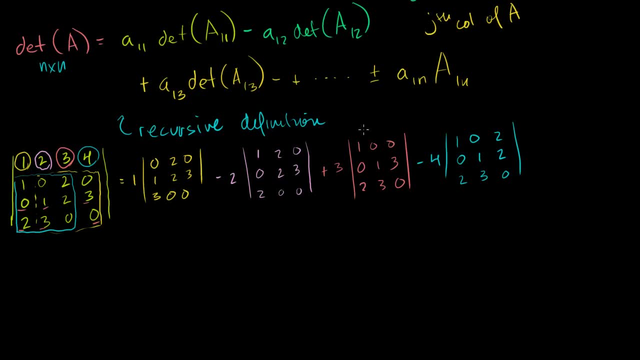 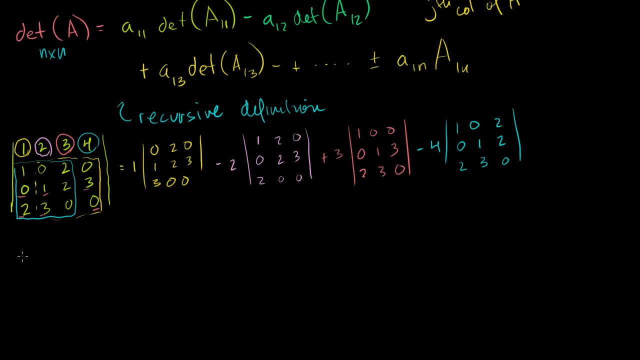 We could use the definition of the 3 by 3, but we could just keep applying this recursive definition. So this is going to be equal to- Let me write it here: So 1 times what's this determinant? This determinant is going to be 0. 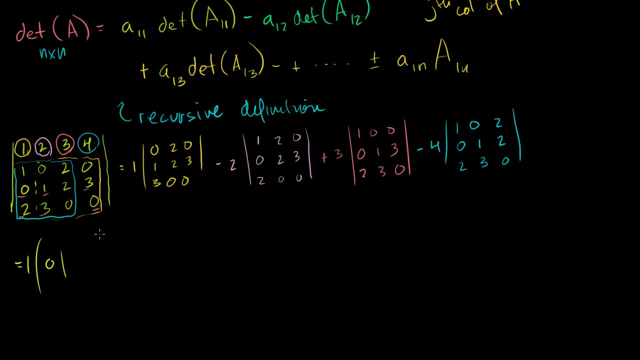 0 times the determinant of that sub-matrix: 2, 3, 0, 0.. 2, 3, 0, 0.. That was this one right here. And then we have minus 2, minus this 2.. 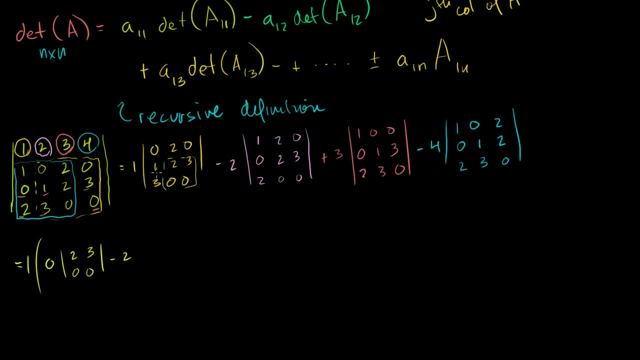 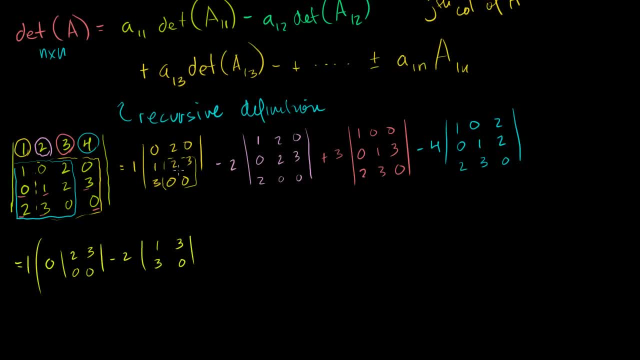 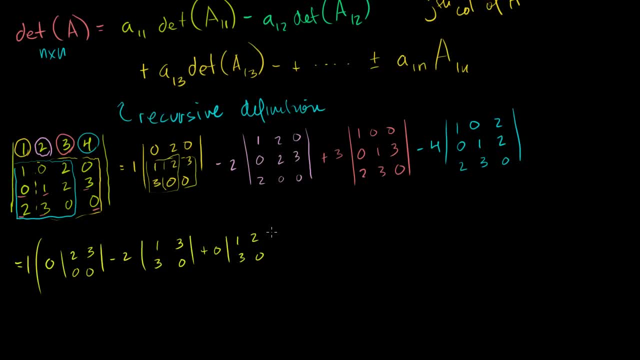 1, 2, 3, 0.. 1, 2, 3, 0.. Just like that, And then we have this next guy right here. As you can see, this can get a little bit tedious, but we'll. 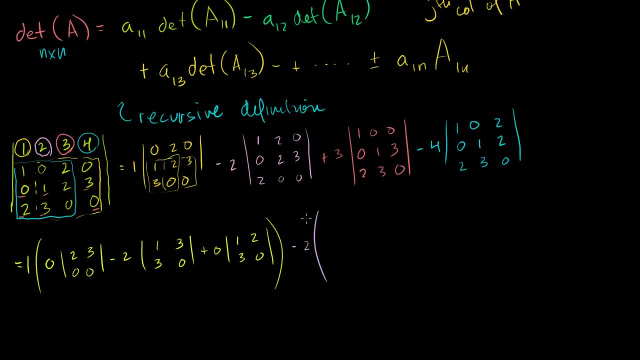 keep our spirits up. So minus 2 times, 1 times its sub-matrix. So that's this guy right here, So that's the determinant of this sub-matrix, of its submatrix 2, 3, 0, 0.. 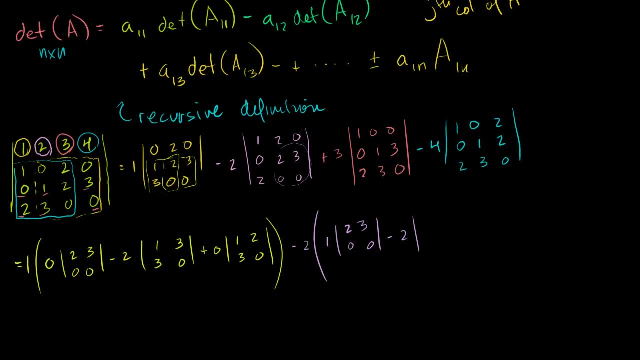 Then minus 2 times, get rid of that row, that column 0, 3, 2, 0, 0, 3, 2, 0.. And then plus 0 times 0, 2, 2, 0, 0, 2, 2, 0.. 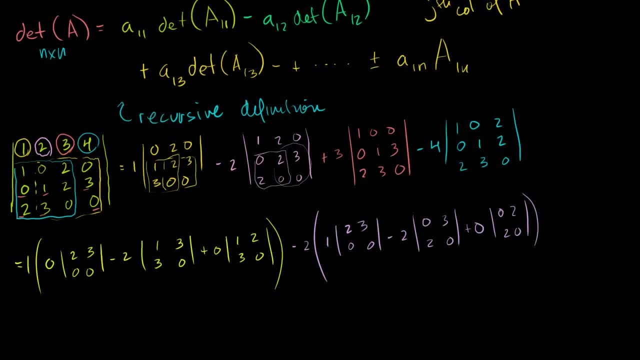 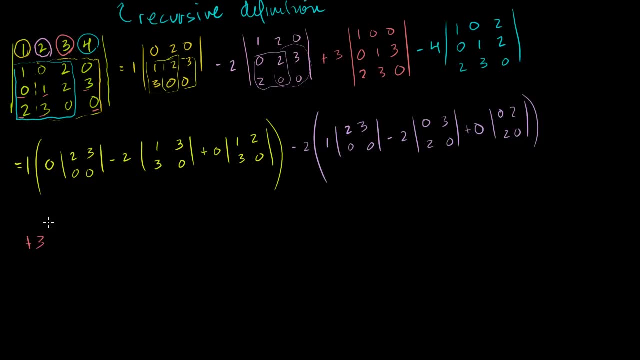 That's this one right there, Halfway there, at least for now, And then we get this next one. So we have a plus 3, bring out our parentheses And then we're going to have 1 times its subdeterminant. 1, 2, 3, 0. 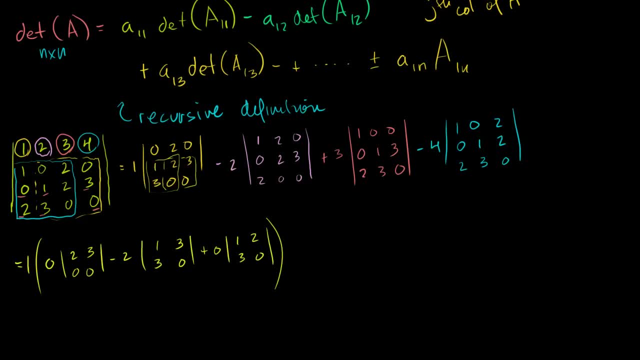 Just like that. And then we have this next guy right here. 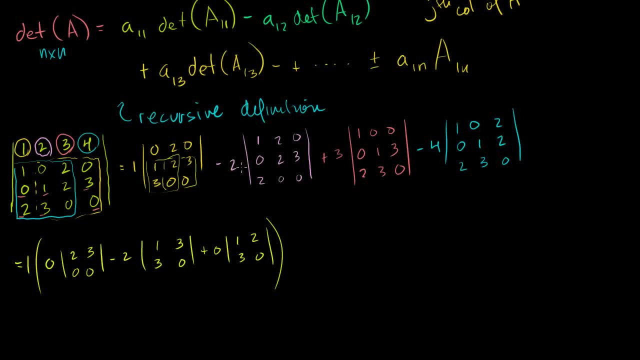 As you can see, this can get a little bit tedious, but we'll keep our spirits up. 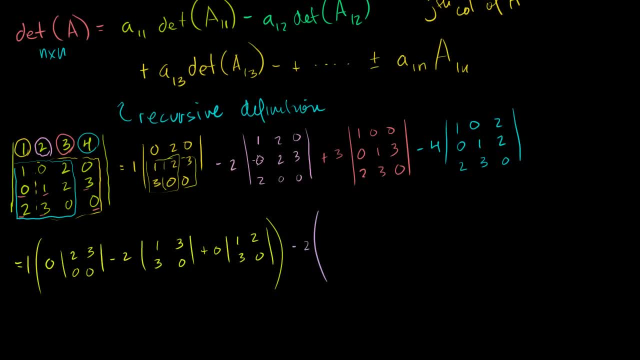 So minus 2 times 1 times its sub matrix. So that's this guy right here. This is the determinant of its sub matrix. 2, 3, 0, 0. 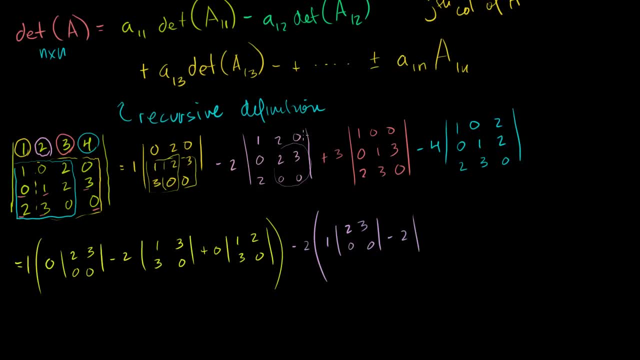 Then minus 2 times, get rid of that row, that column. 0, 3, 2, 0. 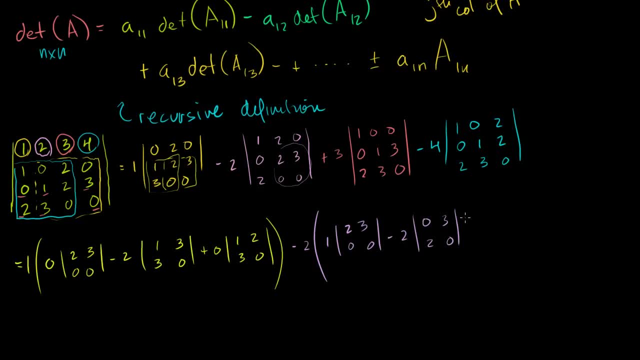 0, 3, 2, 0. And then plus 0 times 0, 2, 2, 0. 0, 2, 2, 0. That's this one right there. 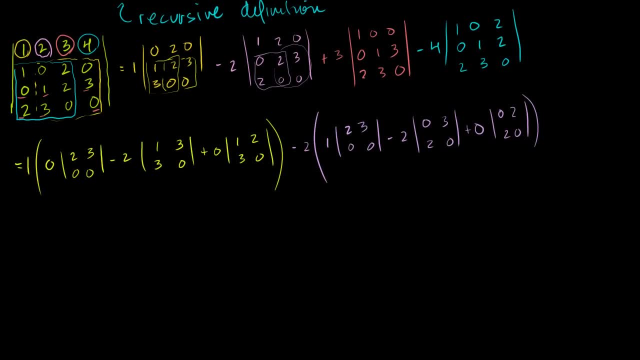 Halfway there, at least for now. And then we get this. Next one. So we have a plus 3. 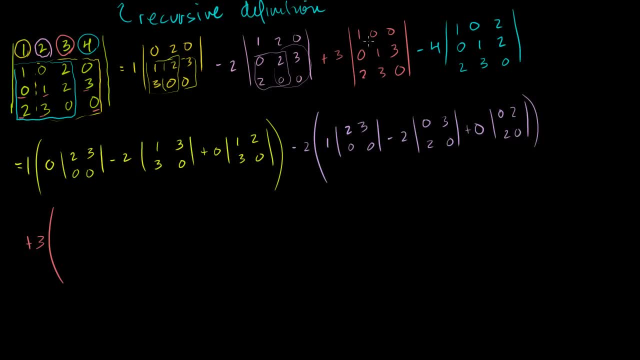 Plus 3. Bring out our parentheses. And then we're going to have 1 times its sub, I guess call it, subdeterminant. So 1 times the determinant 1, 3, 3, 0. You get rid of this guy's row and column. You get this guy right there. And then minus 0, get rid of this row and column, times 0, 3, 2, 0. 0, 3, 2, 0. 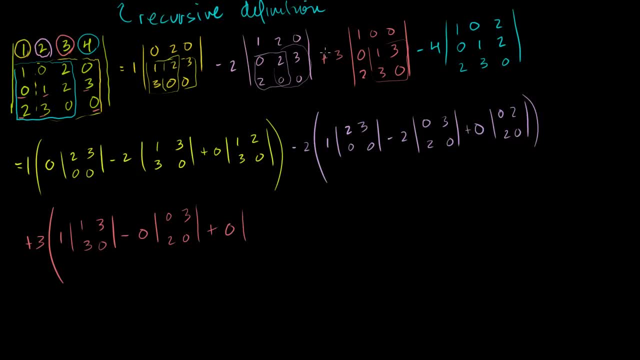 And then you have plus 0. Plus 0 times its subdeterminant. 0, 1, 2, 3. 0, 1, 2, 3. 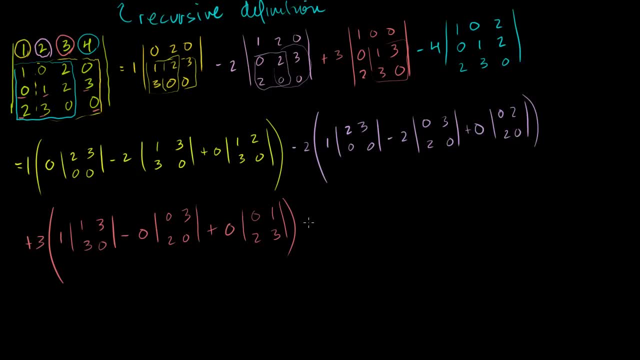 3 fourths of the way there. One last term. Let's hope we haven't made any careless mistakes. 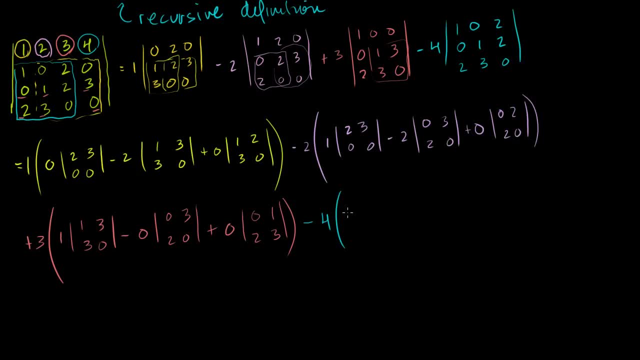 Minus 4 times 1 times 1, 2, 3, 0. 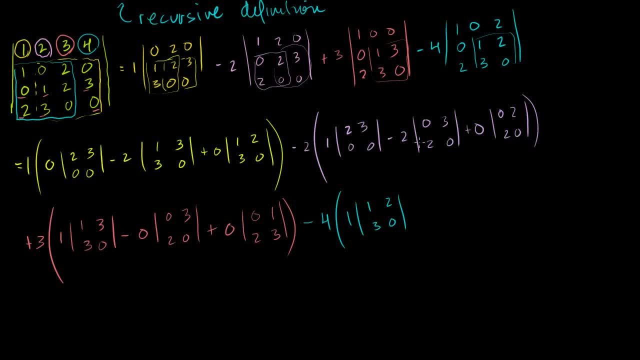 Right there. 1, 2, 3, 0. Minus 0 times, get rid of those two guys. 0, 2, 2, 0. 0, 2, 3, 0. 0, 2, 2, 0. And then plus 2 times 0, 1, 2, 3. Plus 2, get rid of these guys. 0, 1, 2, 3. 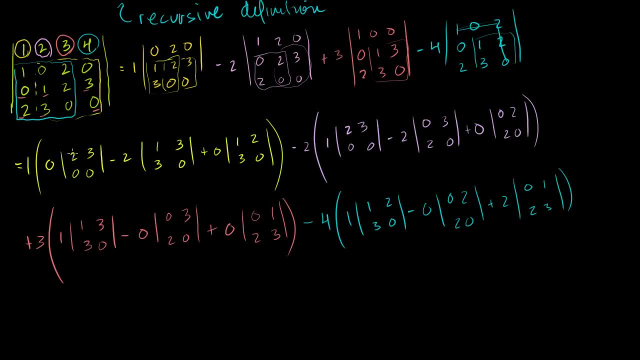 0, 1, 2, 3. Now we've calculated or we've defined our determinant of 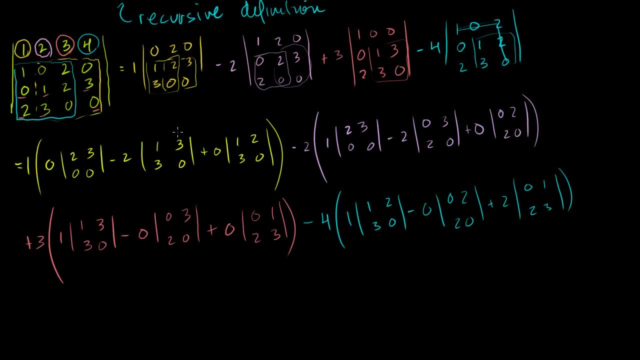 this matrix in terms of just a bunch of 2 by 2 matrices. So hopefully you saw in this example that the recursion worked out. 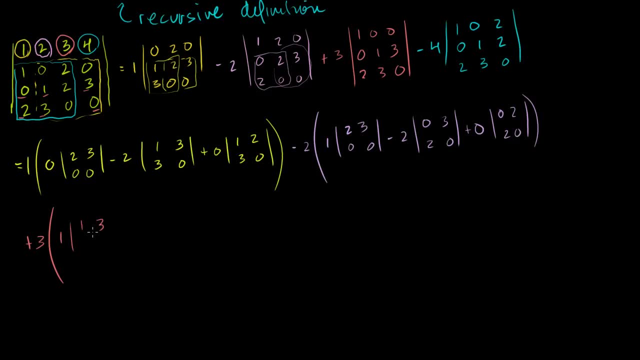 So 1 times the determinant: 1,, 3,, 3,, 0.. You get rid of this guy's row and column, You get this guy right there And then minus 0, get rid of this row and column times 0,. 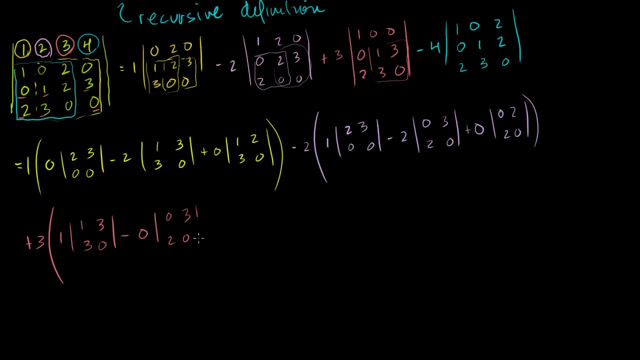 3, 2, 0, 0, 3,, 2, 0.. And then you have plus 0.. Plus 0 times its subdeterminant 0, 1, 2, 3, 0, 1,. 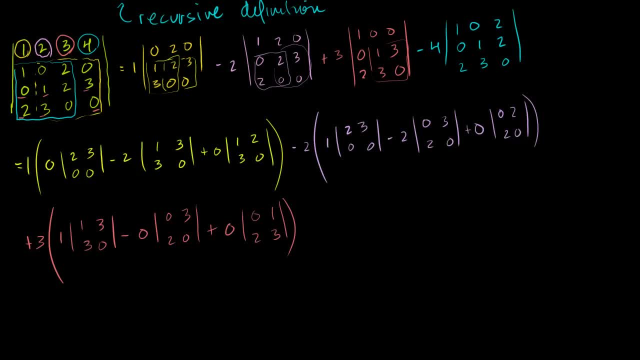 2, 3, 3. fourths of the way there. one last term. Let's hope we haven't made any careless mistakes. Minus 4 times 1 times 1, 2, 3, 0,. right there: 1, 2, 3, 0. 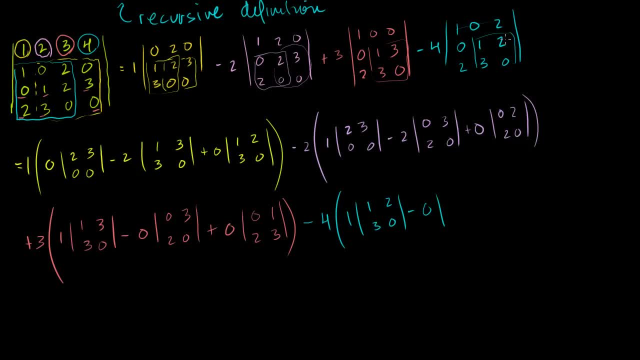 Minus 0 times. get rid of those two guys: 0, 2,, 2,, 0,, 0, 2,, 2, 0, and then plus 2 times: 0,, 1,, 2,, 3, right. 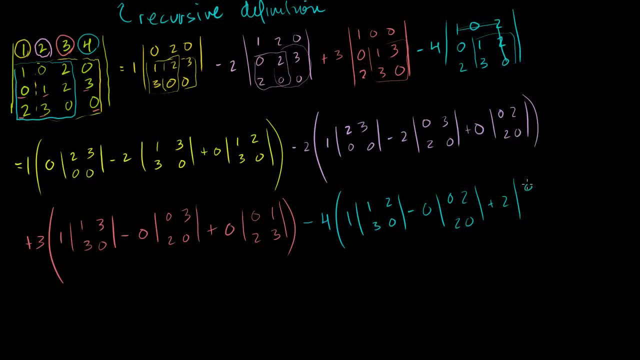 Plus 2, get rid of these guys: 0, 1, 2, 3, 0, 1, 2, 3.. Now we've defined our, or we've calculated, or we've defined our determinant of this matrix in terms of just a bunch of 2. 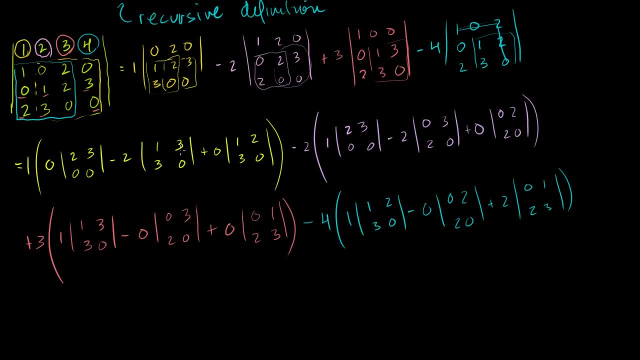 by 2 matrices. So hopefully you saw in this example that the recursion worked out. So let's actually find what this number is equal to. A determinant is always just going to be a number, So let me get a number. OK, Nice, vibrant color. 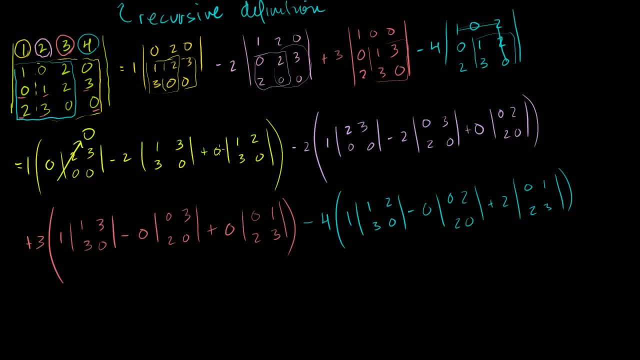 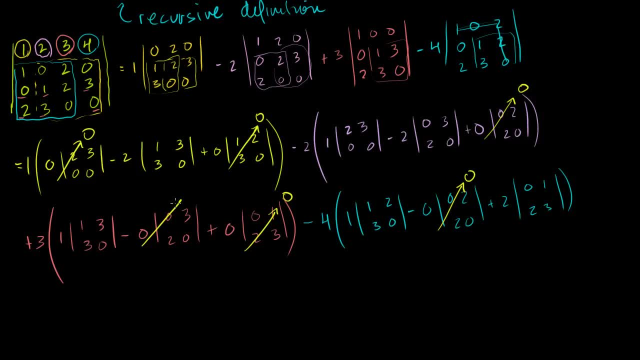 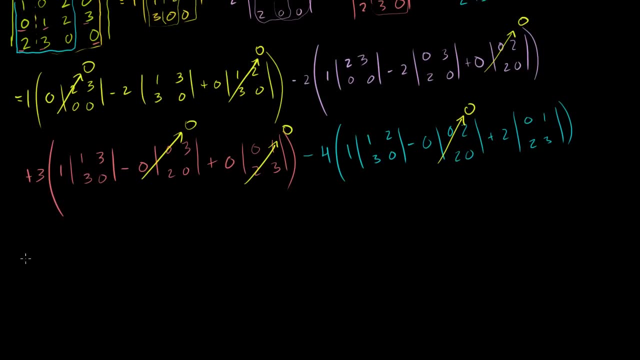 Just simplifying it, these guys are 0, because it's 0 times that. 0 times this is going to be equal to 0. So what are we left with? This is going to be equal to 1 times. this is all we have. 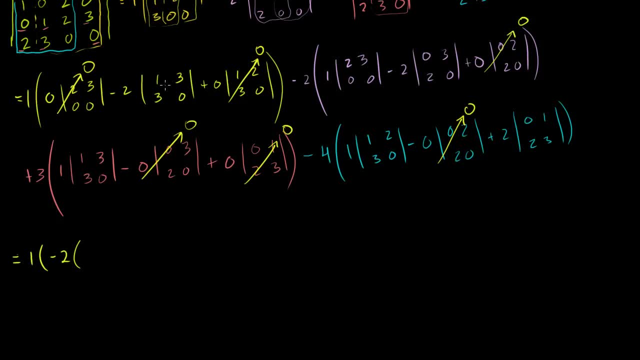 left. here is a minus 2, times, and what does this determine? It's 1 times 0, which is 0.. It's 0,. let me write this: This is going to be 1 times 0, 0 minus 3 times 3, 0 minus 9.. 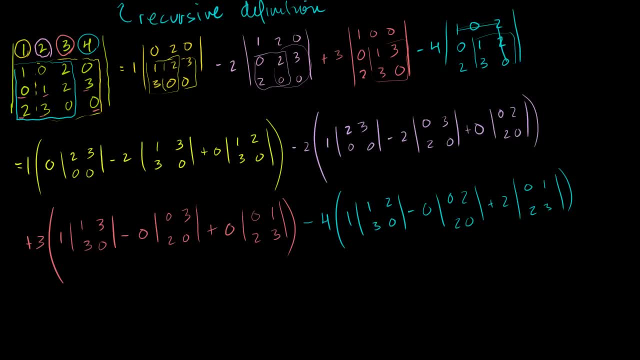 So let's actually find what this number is equal to. A determinant is always just going to be a number. 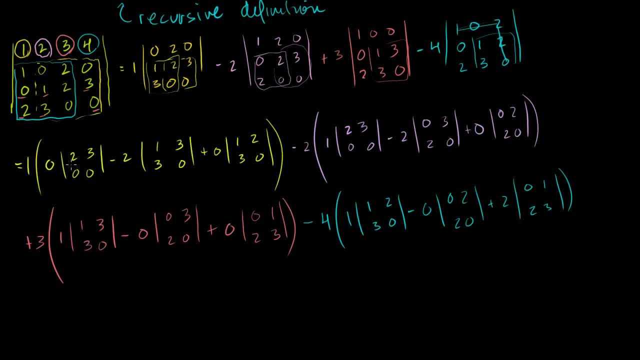 So let me get a nice vibrant color. So this is a 0 times, I don't care, 0 times anything is going to be 0. 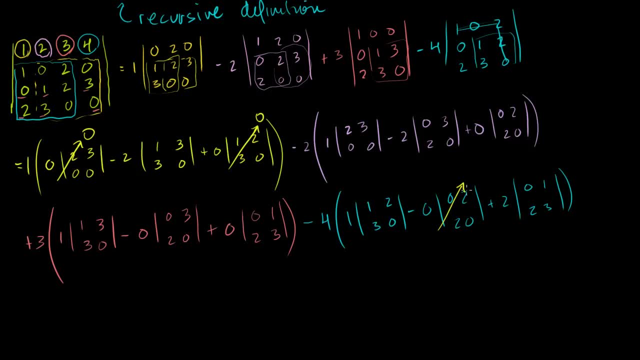 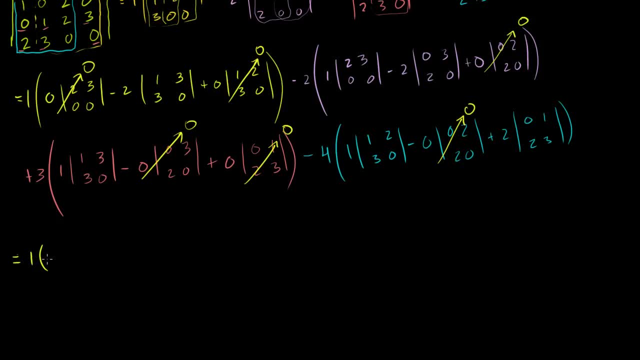 This is going to be equal to 1 times, this is all we have left here is a minus 2. 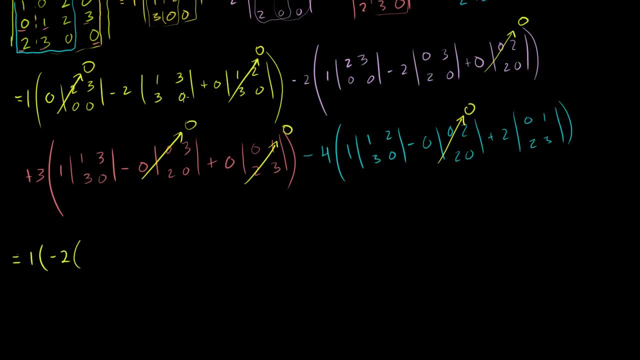 Times, and what does this determine? It's 1 times 0, which is 0. 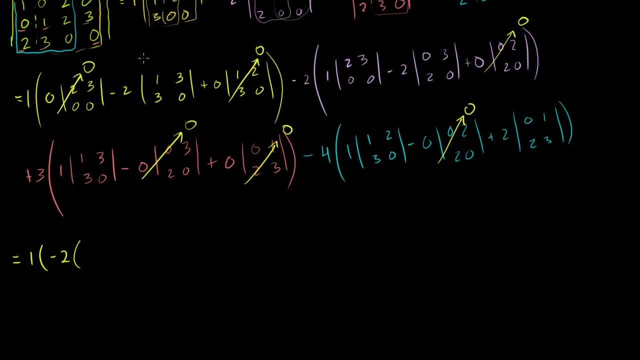 It's 0, let me write this. This is going to be 1 times 0, 0 minus 3 times 3, 0 minus 9. So minus 9. This right here is just minus 9. So minus 2 times minus 9. That's our first thing. I'll simplify it in a second. 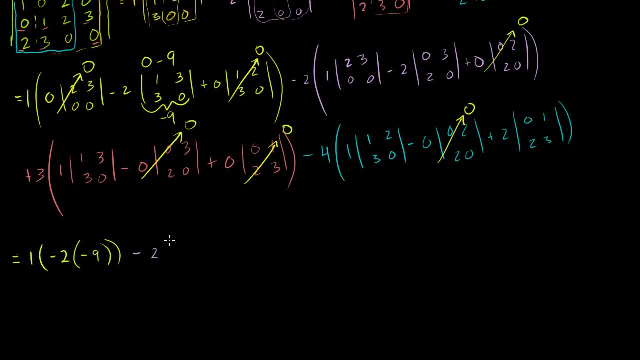 Now let's do this term right here. So it's minus 2 times. Now what's this determinant? 2 times 0. Minus 0 times. 0 times 3, that's 0 minus 0, so this is 0. That guy became 0, so we can ignore that term. This term right here is 0 times 0, which is 0, minus 2 times 3, so it's minus 6. 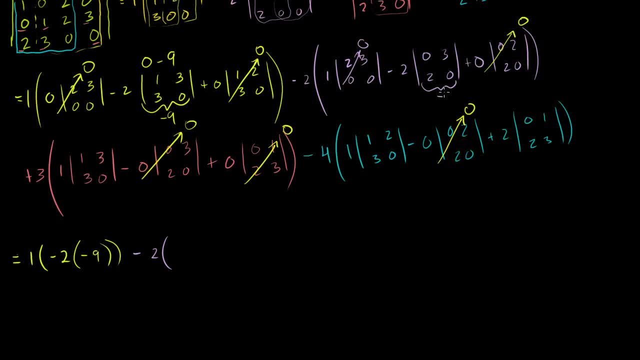 So it's minus 2 times, so this is a minus 6 right here. You have a minus 2 times a minus 6, so that's a plus 12. So I'll just write a plus 12 here. This minus 2 is that minus 2 right there. And then we have a plus 3. We have this plus 3. And then this first term is 1 times 0, which is 0, minus 1 times 0, which is 0, minus 3 times 3, which is minus 9, times 1, so it's minus 9. Everything else was a 0. We're in the home stretch. 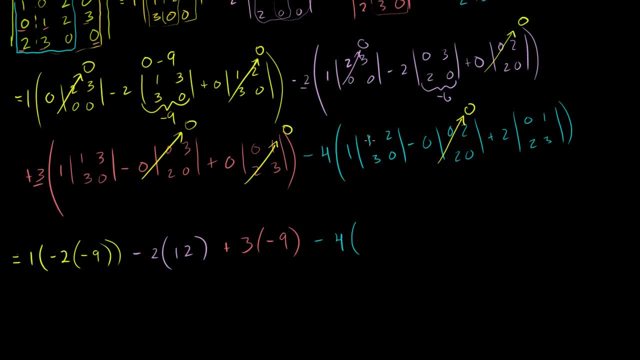 We have a minus 4. Let's see, this is 1 times 0, which is 0, minus 3 times 2, so minus 6. So this is minus 6 right here. Minus 6. This is 0. And then we have this guy right here. 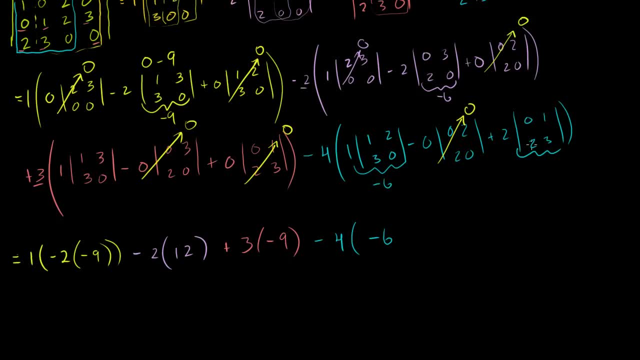 So we have 0 times 3, which is 0, minus 2 times 1, so that's minus 2. 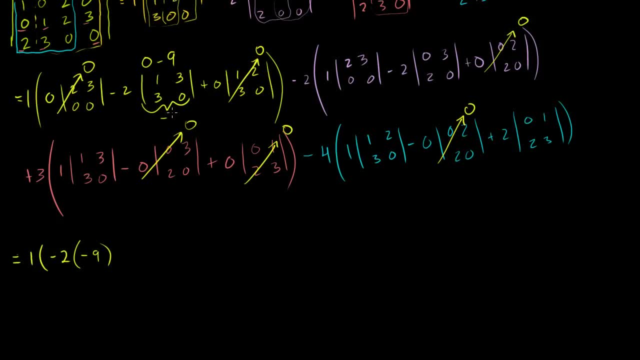 So minus 9.. This right here is just minus 9.. So minus 2 times minus 9.. That's our first thing. I'll simplify it in a second. Now let's do this term right here. So it's minus 2 times. 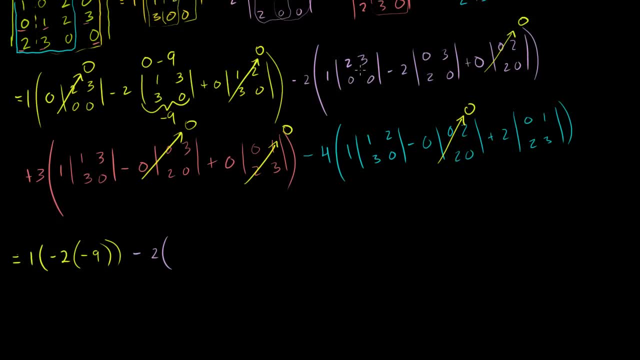 Now what's this determinant? 2 times 0 minus 0, times 3.. 0 minus 0,, so this is 0.. That guy became 0, so we can ignore that term. This term right here is 0 times 0, which is 0, minus 2 times. 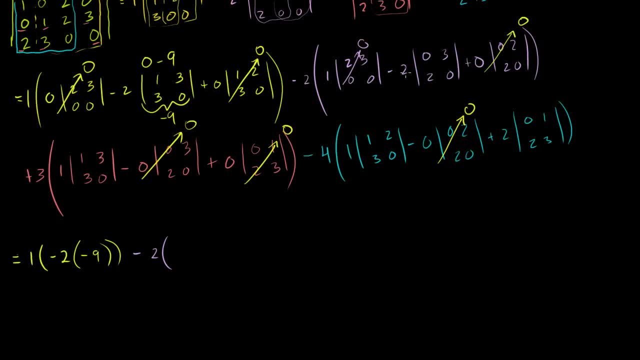 3,, so it's minus 6.. So it's minus 2 times. so this is a minus 6, right here. So you have a minus 2 times a minus 6, so that's a plus 12.. So I'll just write a plus 12 here. 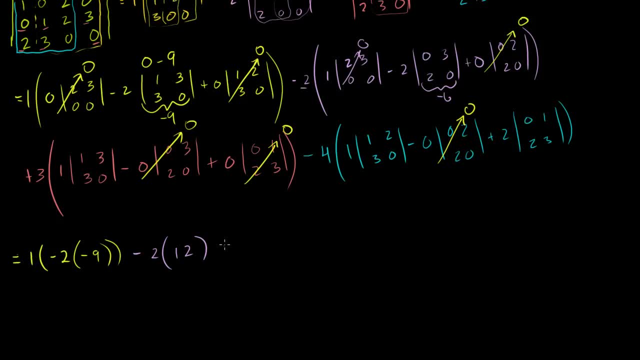 This minus 2 is that minus 2 right there, And then we have a plus 3.. We have this plus 3, and then this first term is 1 times 0,, which is 0, minus. let me make a parenthesis here. 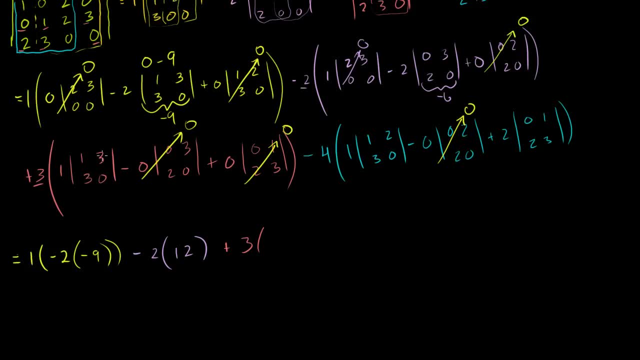 1 times 0,, which is 0,, minus 3 times 3,, which is minus 9, times 1,, so it's minus 9.. Everything else was a 0.. We're in the home stretch. We have a minus 4.. 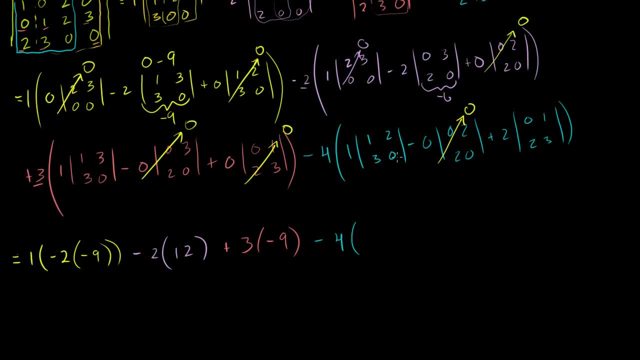 Let's see, this is 1 times 0,, which is 0, minus 3 times 2,, so minus 6.. So this is minus 6, right here, Minus 6.. This is 0.. And then we have this guy right here. 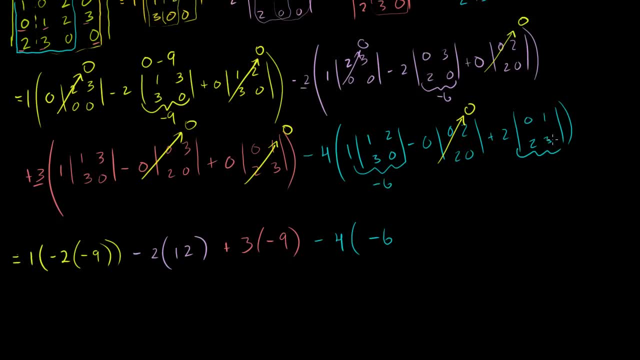 So we have 0 times 3,, which is 0, minus 2 times 1,, so that's minus 2.. And then you have a minus 2 times a plus 2,- it's minus 4.. So now we just have to make sure we do our arithmetic. 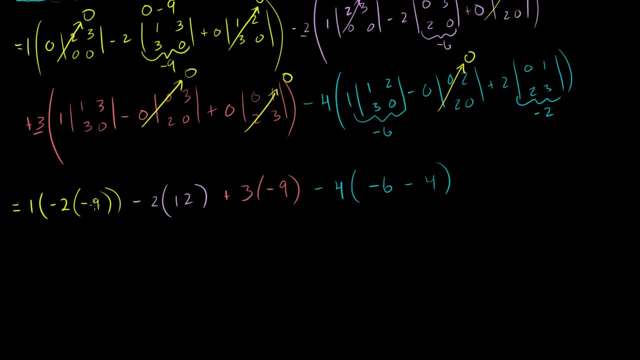 properly, This is 1 times plus 18, so this is 18, right Minus 2 times minus 9.. This right here is minus 24.. This right here is minus 18.. This right here is minus 24.. 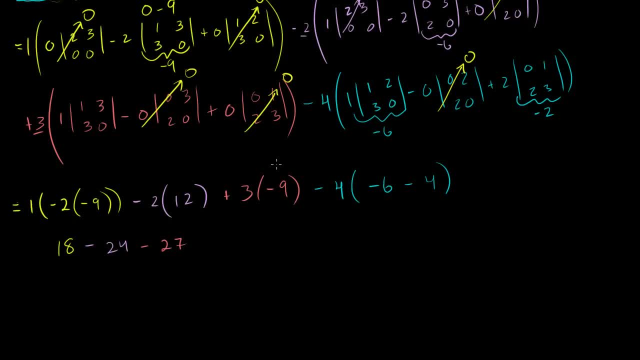 This right here is minus 27.. And then this right here: let's see, this is minus 10. right here, that is minus 10.. Minus 4 times minus 10 is plus 40. Plus 40. And let's see if we can simplify this a little bit. 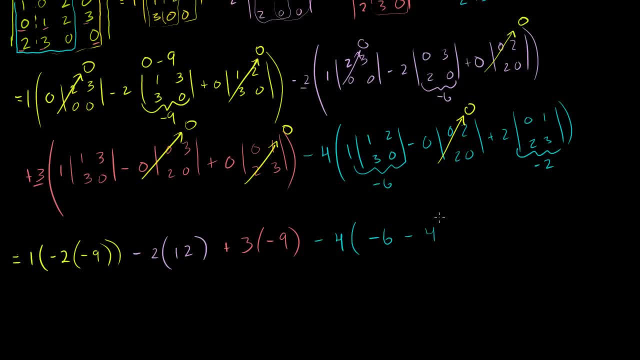 And then you have a minus 2 times a plus 2, so it's minus 4. 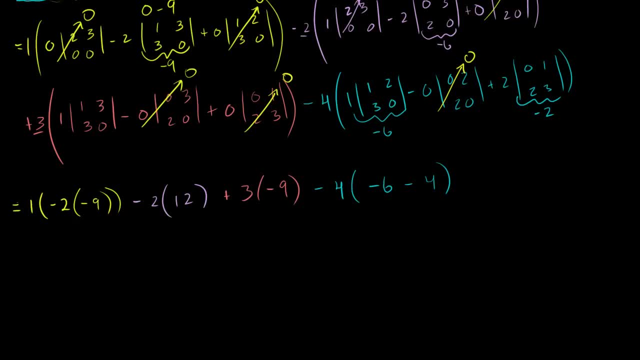 So now we just have to make sure we do our arithmetic properly. 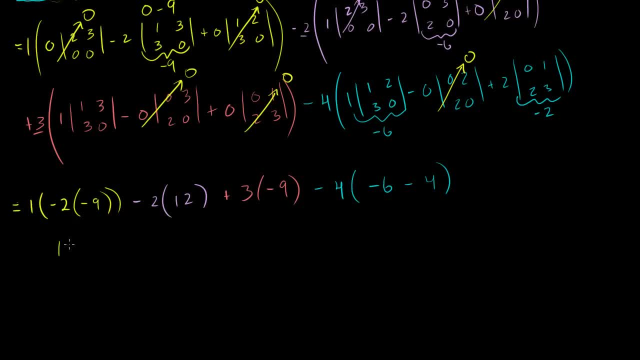 This is 1 times plus 18, so this is 18, right? Minus 2 times minus 9. 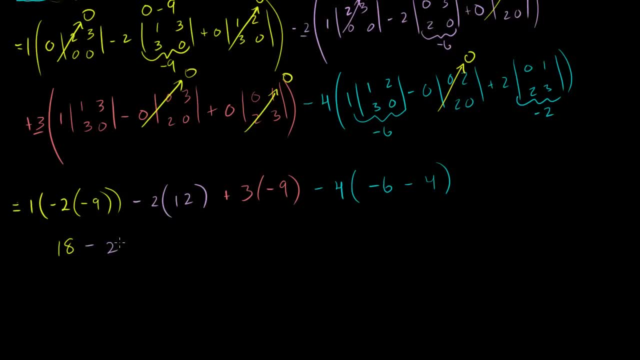 This right here is minus 24. 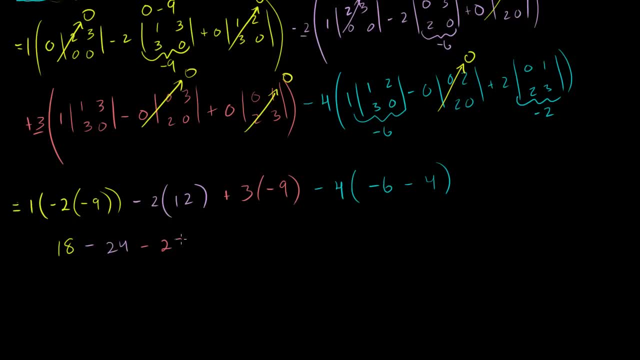 This right here. This right here is minus 27. 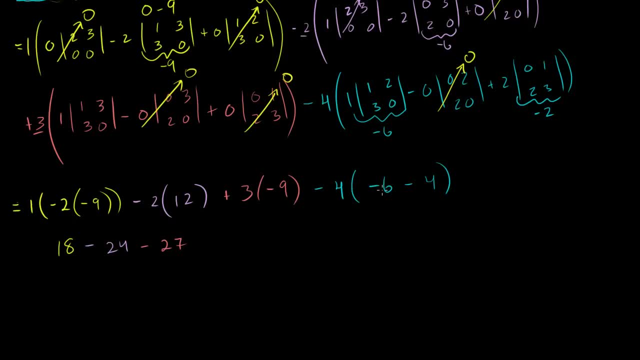 And then this right here, let's see, this is minus 10 right here, that is minus 10. 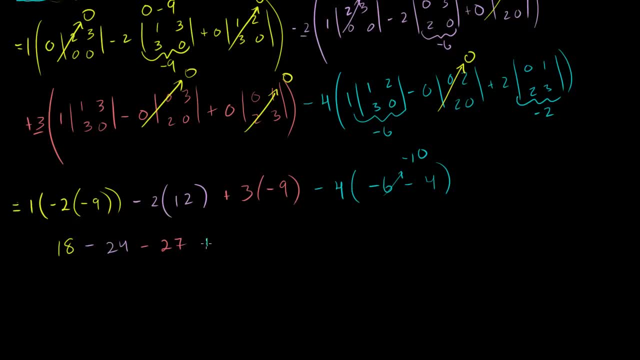 Minus 4 times minus 10 is plus 40. Plus 40. 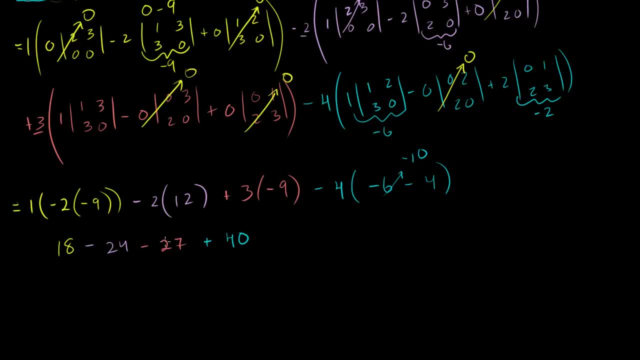 Plus 40. And let's see if we can simplify this a little bit. If we simplify this a little bit. 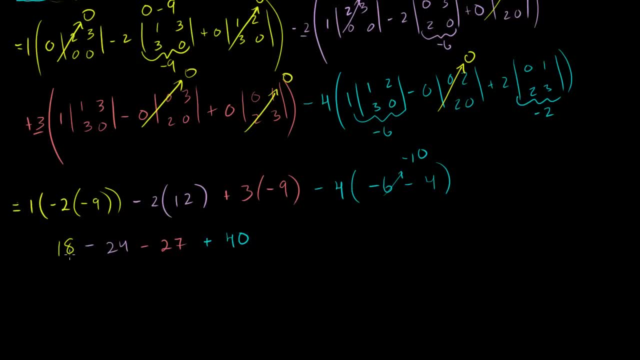 I don't want to make a careless mistake right at the end. So 18 minus 24. 18 minus 24. 24 minus 18 is 6. So this is going to be equal to minus 6, right?